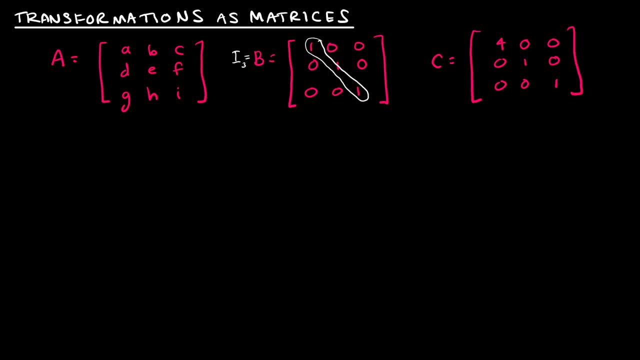 is made up of a diagonal of ones with all other values. that was a horrible circling, with all other values being zero, and the whole point is, if I take that identity matrix times any other matrix, and we're actually going to multiply this out just for fun- 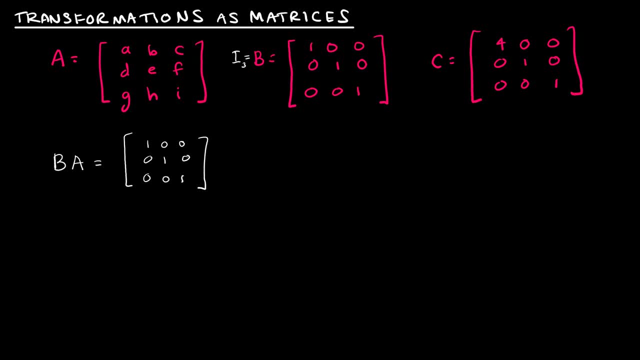 because who doesn't love multiplying matrices? and hopefully, before I even start multiplying this out, you're saying, Professor Brame, don't waste my time. I already know what the result is going to be. and that's true. hopefully you do, because that's the point of the identity matrix. but let's take 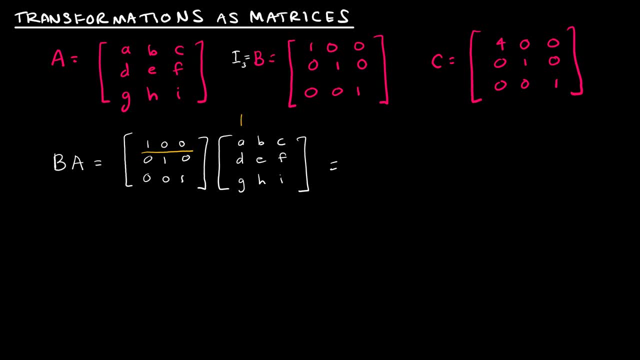 one zero zero times my first column, so I'll get one a plus zero d plus zero g, so that's a, and then times the next column, I would get one b plus zero e plus zero h, and then times the next column and I would get one c plus zero, f plus zero i. 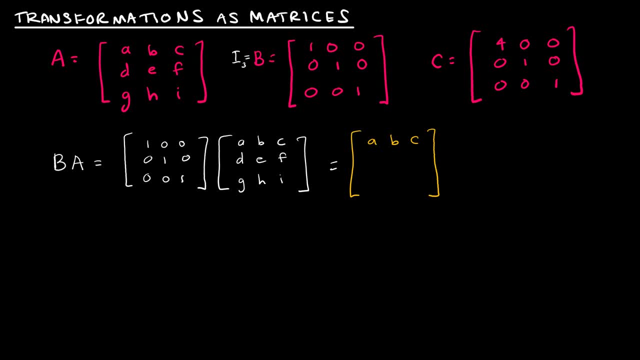 and then I would move on to my next row: zero one zero, so zero a plus one d plus zero g, and hopefully we're sensing the pattern here and, like I said, this should have been the pattern that you knew was going to occur before I ever even started multiplying. 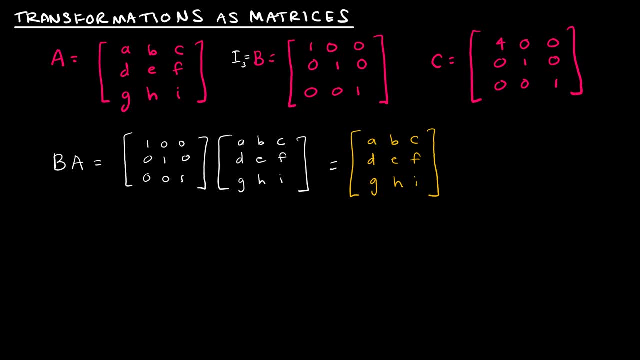 because the whole point of multiplying by the identity matrix is, of course, that I end up back where I started, and that's what I did and notice I did the left multiplication here, and the reason I point that out is because with matrices we know it's important the order in which we multiply things. 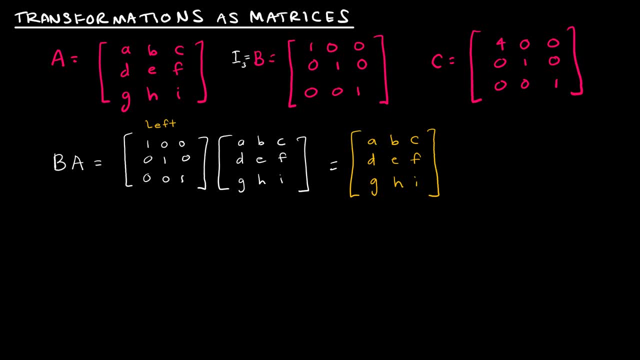 multiplication is not commutative. so that's what I did now and you'll see that the equation is linked to the basis here, because I know it's important- the order in which we multiply things. multiplication is not commutative. Now, knowing what just happened, I 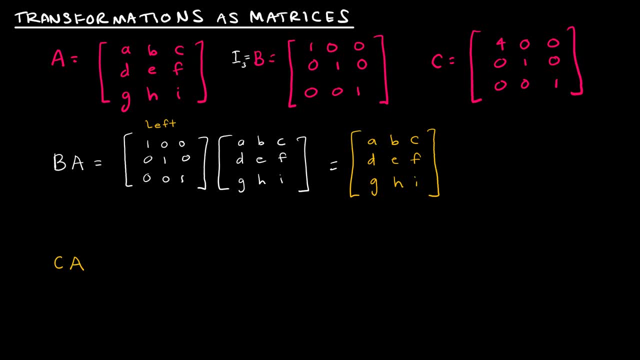 want you to take a guess at what will occur when I take c times a. So be thinking about that while I copy c and a. So any guesses? What do you think is going to happen when I multiply c times a? So the only difference between b and c is that c has a 4,. 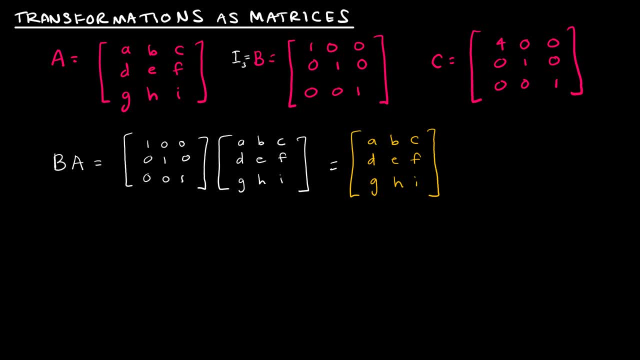 because the whole point of multiplying by the identity matrix is, of course, that I end up back where I started, and that's what I did notice. I did the left multiplication here, and the reason I point that out is because with matrices we know it's important the order in which we multiply things. 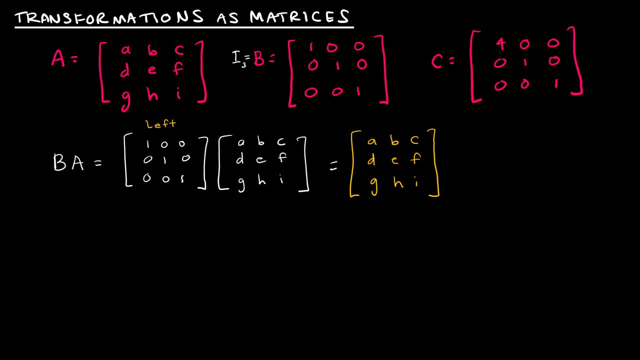 multiplication is not commutative. Now, knowing what just happened, I want you to take a guess at what will occur when I take C times A. So be thinking about that while I copy C and A. So any guesses? What do you think is going to happen when I multiply C times A? 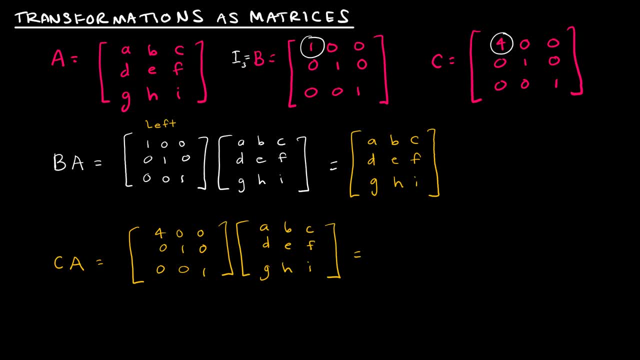 So the only difference between B and C is that C has a 4, where B has a 1 in that first row. So my guess is something's going to get multiplied by 4, and hopefully you are being more specific than something. 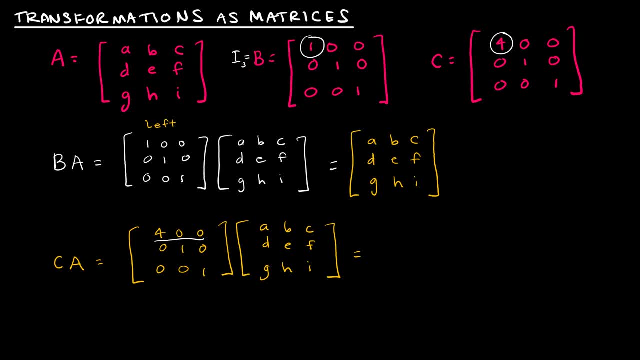 But let's go ahead and see what happens. So I'm going to take 4, 0, 0, times A, D, G, So that first row times the first column And notice what I get is 4A plus 0D plus 0C. 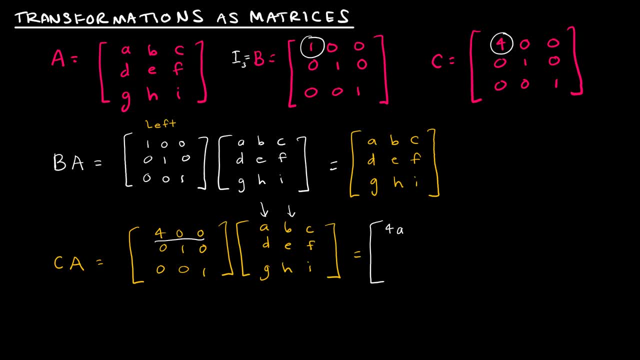 So that's 4A, And then times the next column 4B plus 0E plus 0H, So that's 4B, And then times the next column and I get 4C plus 0F plus 0I. 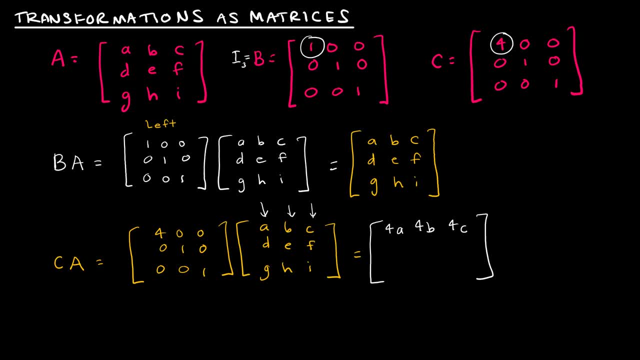 And then moving on to the next two rows, obviously- and I'm not going to multiply those out, because I already did on my last question- and those two didn't change- Those two rows were exactly the same As they were up here. 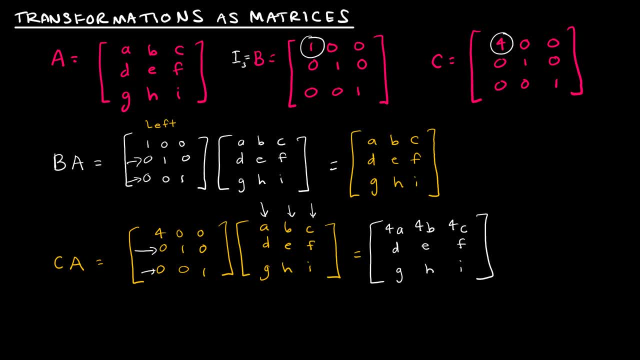 So what happened when I made that a 4?? Is there some sort of row operation that we know? Let's just put it. instead of an equal sign, Let's say: what row operation did I use to get from? well, I don't want to make things confusing. 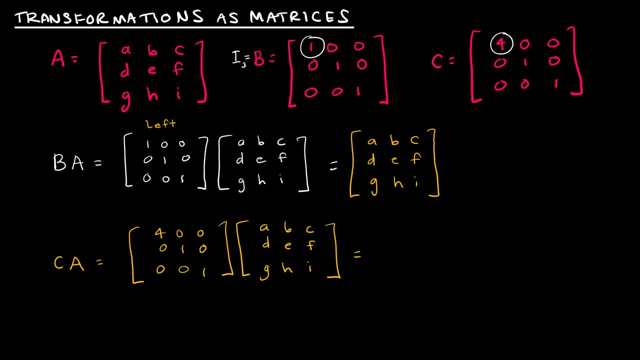 where b has a 1 in that first row. So my guess is: something's going to get multiplied by 4, and hopefully you are being more specific than something, But let's go ahead and see what happens. So I'm going to take 4, 0, 0 times a, d, g. 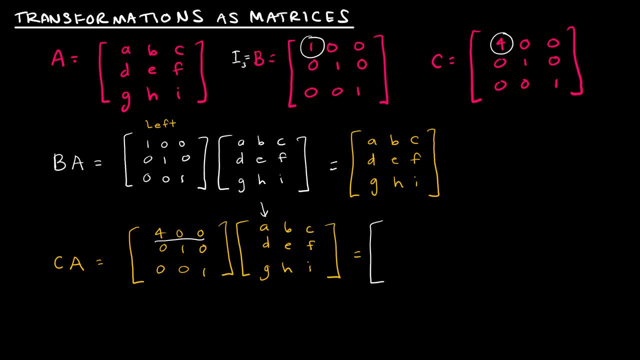 So that first row times the first column And notice what I get is 4a plus 0d plus 0g, So that's 4a, And then times the next column: 4b plus 0e plus 0h. 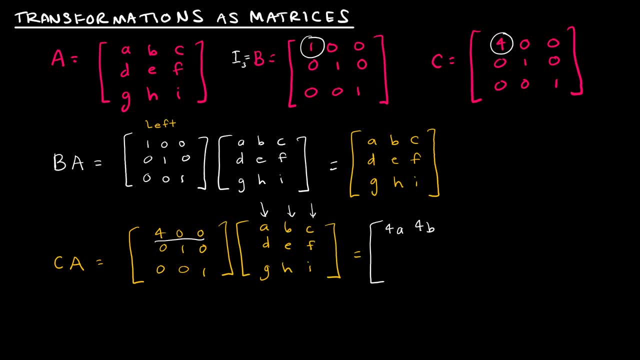 So that's 4b, And then times the next column and I get 4c plus 0f plus 0i, And then moving on to the next two rows, obviously, and I'm not going to multiply those out because I already- 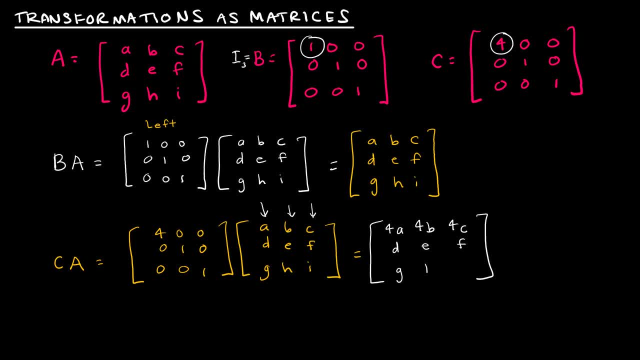 did on my last question, and those two didn't change. Those two rows were exactly the same As they were up here. So what happened when I made that a 4?? Is there some sort of row operation that we know? Let's just put it instead of an equal sign. 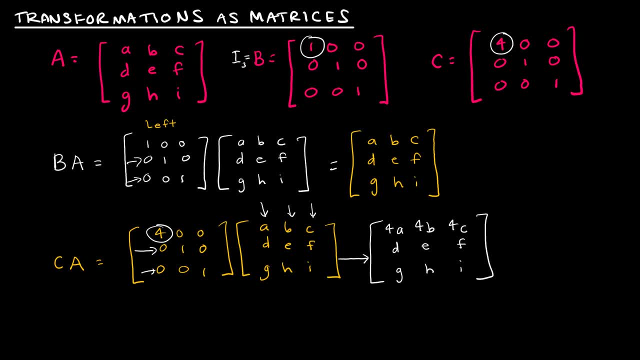 Let's say: what row operation did I use to get from? Well, I don't want to make things confusing, Let's just recopy this: a, b, c, d, e, f, g, h, i. What row operation would I use to get to? 4a, 4b, 4c. 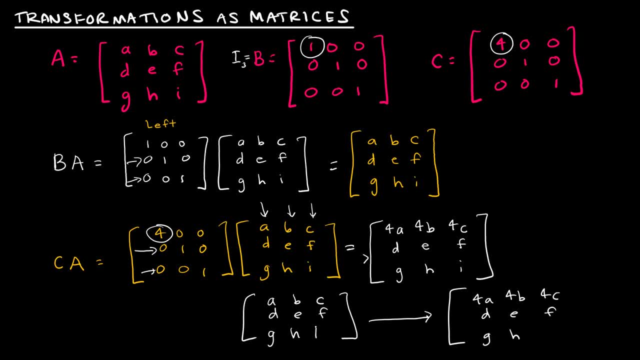 d, e, f, g, h, i And hopefully we can say: well, if I took 4 times row one, that would be my new row one. So this obviously is a row operation that is equivalent to this matrix. 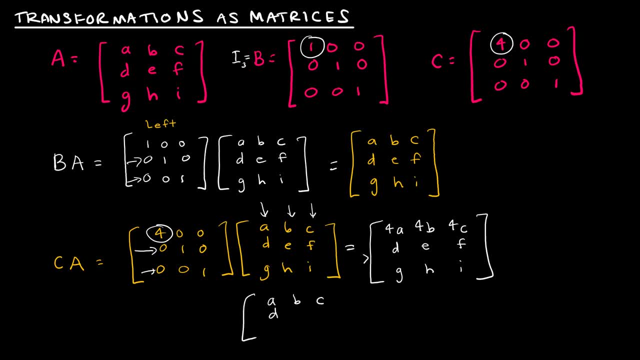 Let's just recopy this: A, B, C, D, E, F, G, H, I. What row operation would I use to get to 4A, 4B, 4C, D, E, F, G, H I? 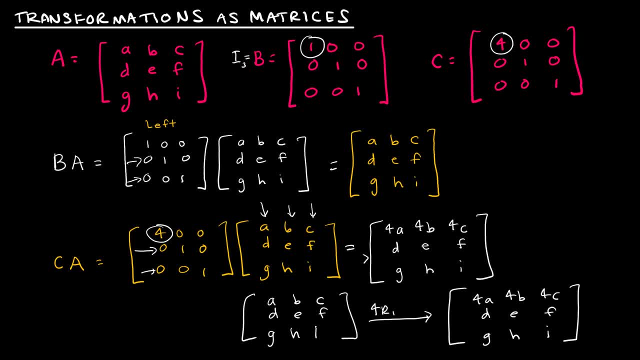 And hopefully we can say: well, if I took 4 times row 1, that would be my new row 1.. So this obviously is a row operation that is equivalent to this matrix And that is a transformation, because we know that these are just transformations. 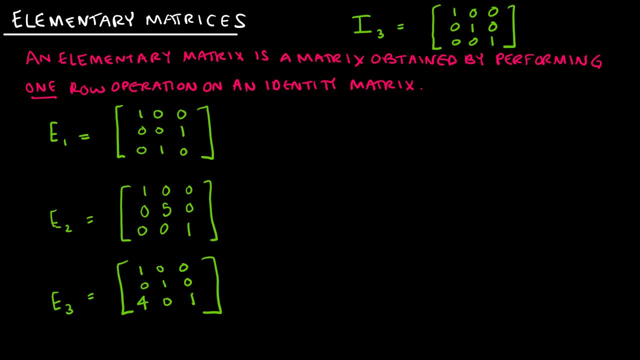 So, now that we're reminded about that relationship that exists between the row operations and the matrix, and what transformation that is, let's take a look at what an elementary matrix is. An elementary matrix is a matrix obtained by performing only one row operation on an identity matrix. 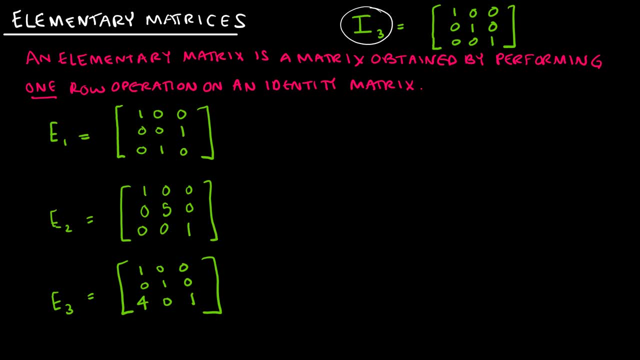 So again, I've rewritten that identity matrix for you up here, because I'm just dealing with 3x3s at this point. And now let's take a look at E1.. What row operation is that equivalent to? Well, I can see that these two rows seem to have been swapped. 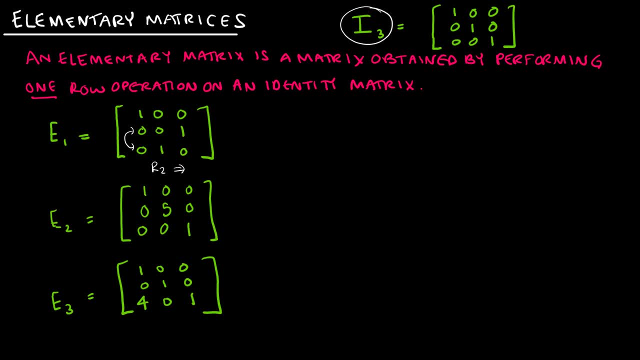 And so that means row 2 was swapped with row 3.. Okay, So if I want to undo that, how am I going to do that? And again, if you need to take this times: A, B, C, D, E, F, G, H, I. 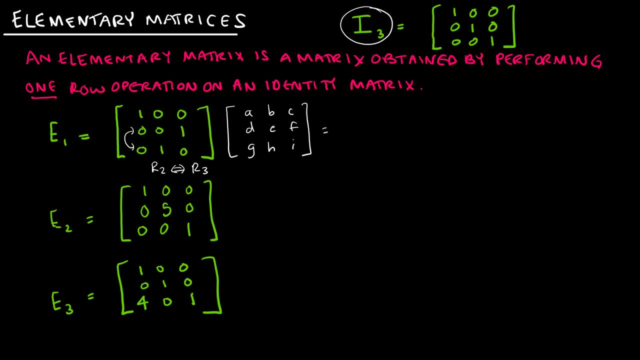 to help you understand what happened. I would get A, B, C and I would get 0A plus 0D plus 1G, And then I would get 0C, 0B plus 0E plus 1H and 0C plus 0F plus 1I, and then I would get 0A plus 1D plus 0G. 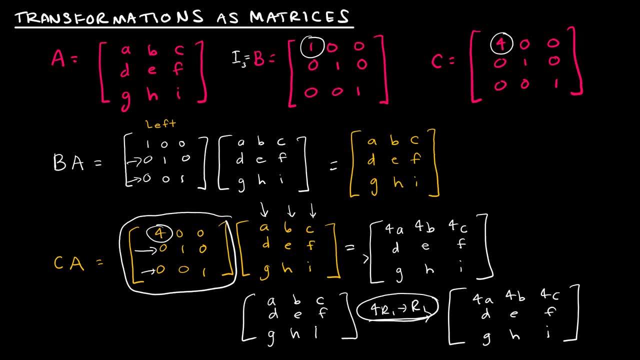 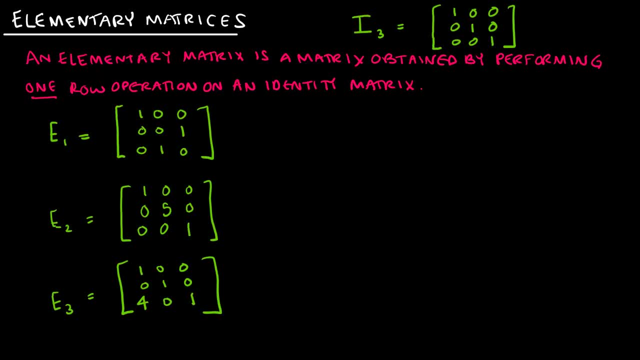 Yeah, Yeah, Yeah, And that is a transformation, because we know that these are just transformations. So, now that we're reminded about that relationship that exists between the row operations and the matrix, and what transformation that is, let's take a look at what an elementary matrix is. 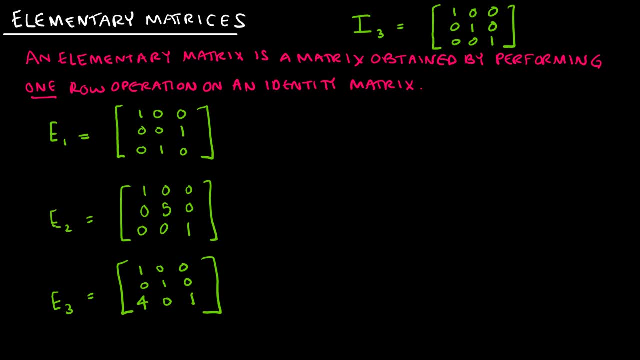 An elementary matrix is a matrix obtained by performing only one row operation on an identity matrix. So again, I've rewritten that identity matrix for you up here, because I'm just dealing with 3x3s at this point. And now let's take a look at E1.. 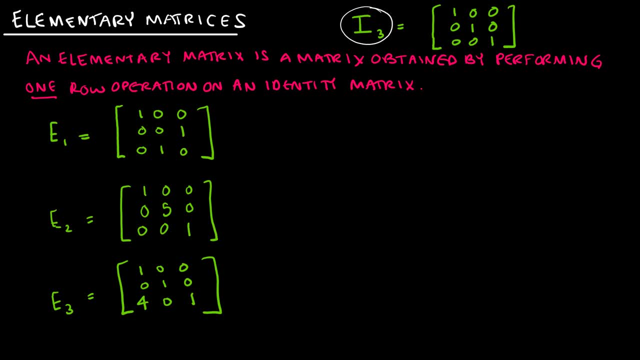 What row operation is that equivalent to? Well, I can see that these two rows seem to have been swapped, And so that means row 2 was swapped with row 3.. So, if, If I want to undo that, how am I going to do that? 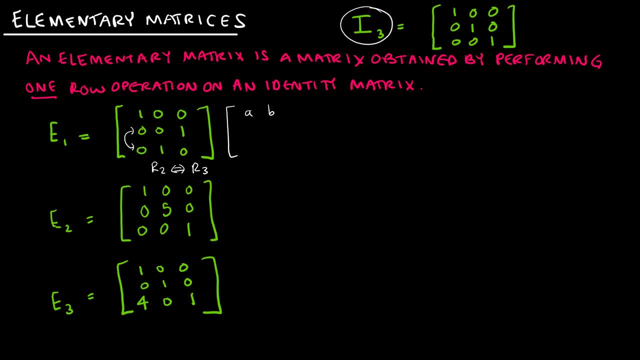 And again, if you need to take this times a, b, c, d, e, f, g, h, i to help you understand what happened, I would get a b c and I would get 0a plus 0d plus 1g. 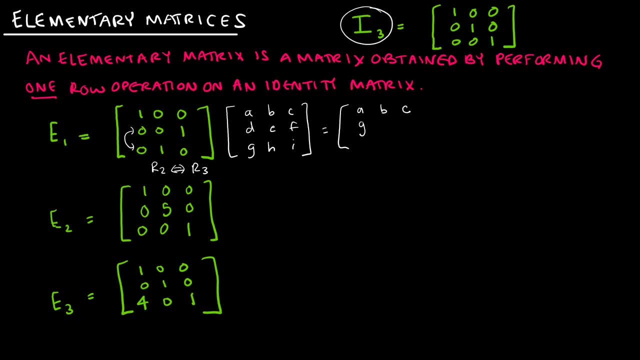 And then I would get 0b Plus 0e plus 1h and 0c plus 0f plus 1i, And then I would get 0a plus 1d plus 0g, And so you get the idea that that's what would happen. is that? sorry that swapped those two rows. 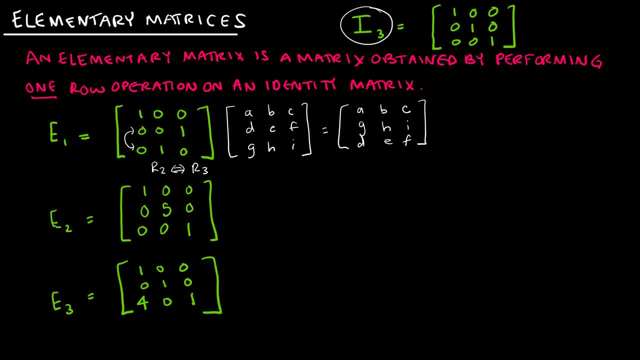 So if I want to undo that, what would I then left? multiply by this guy To get back here- And by that I mean what is the inverse of this guy, Because we know the inverse means undo it. So to get back from this matrix, back to where I started, I would then multiply again by this matrix. 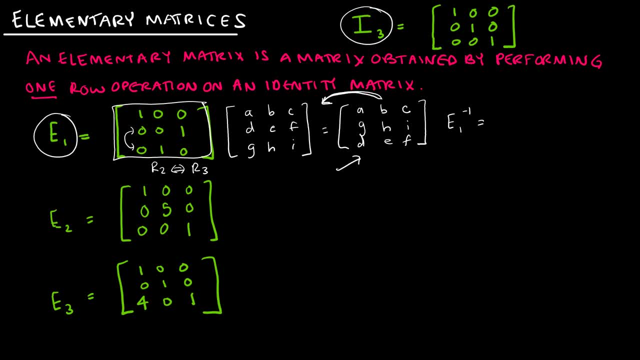 So E1 inverse And E just means that it's an elementary matrix. E1 inverse is E1 inverse is 1, 0, 0, 0, 0, 1, 0, 1, 0.. 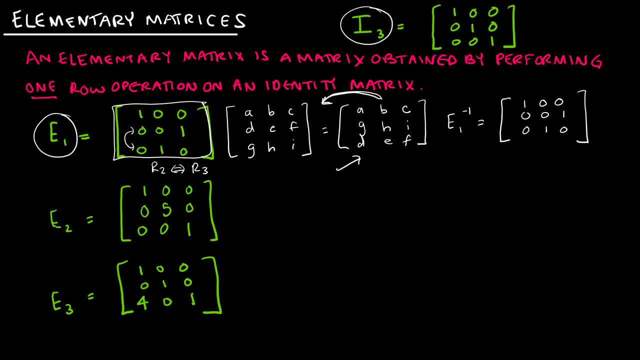 And again, that means, if I took that matrix and I multiplied it 0, 0, 1, 0, 1, 0.. And I multiply it by a, b, c, g, h, i, d, e, f. 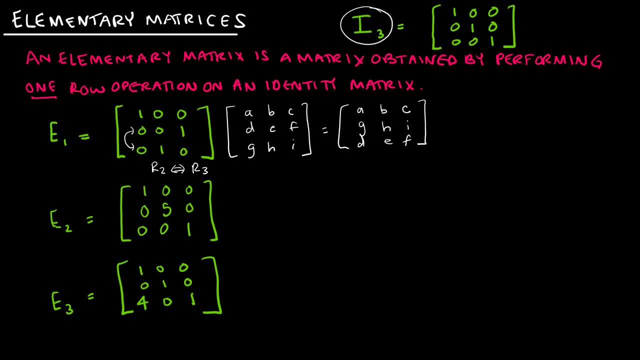 and so you get the idea that that's what would happen. is that? sorry that swapped those two rows. So if I want to undo that, what would I then left? multiply by this guy to get back here, And by that I mean what is the inverse of this guy, Because we know the inverse means. 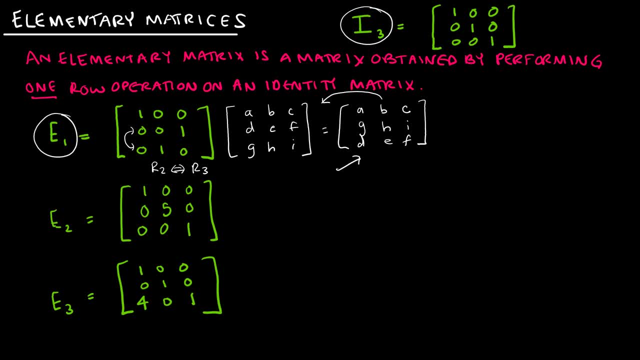 undo it. So to get back from this matrix back to where I started, I would then multiply again by this matrix. So E1 inverse and E just means that it's an elementary matrix- E1 inverse is 1, 0, 0, 0, 0, 1, 0, 1, 0. 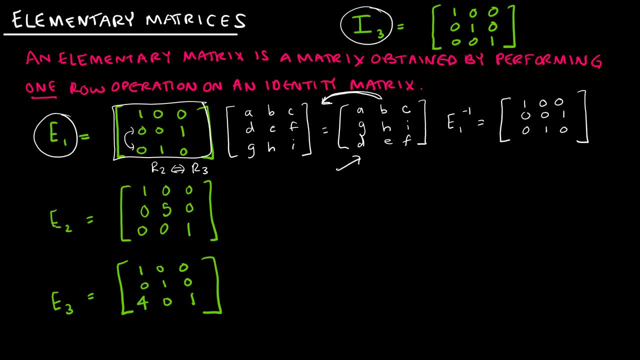 And again, that means, if I took that matrix and I multiplied it 0, 0,, 1, 0, 1, 0, and I multiply it by A, B, C, G, H, I, D, E, F. 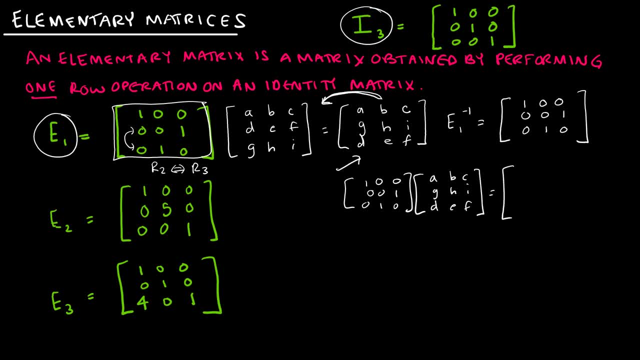 I shouldn't end up with A, B, C, D, E, F, G, H, I and I in fact do So. the inverse again brings us back to where we started, So I'm going to erase this, because I don't. 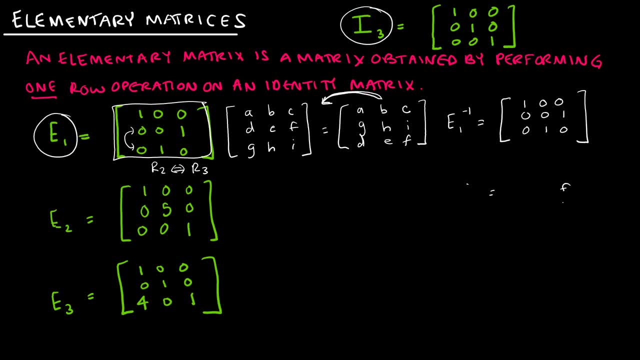 have enough room to show everything All right. so now let's take a look and again, the row operation that would switch it, Of course, just row 3 swapped with row 2, or row 2 swapped with row 3.. 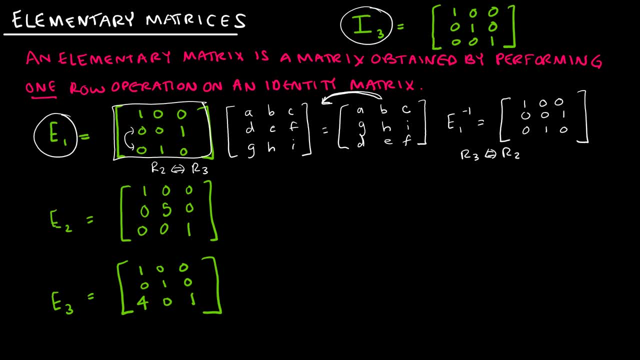 Looking at E2, what would happen? This one we should be familiar with because this is very similar to our last example on the previous slide. This is obviously 5 times row 2 would be my new row 2.. Everything else remained the same And again, notice, that's just one row operation. 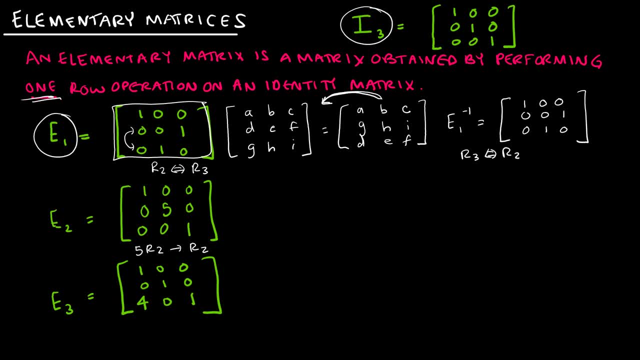 that's happening And I'm not going to multiply it. I'm going to multiply it by A, B, C, D, E, F, etc. We already know what's going to happen. We know that that second row is going to end up being 5,, 5, and 5.. And hopefully you know that already. 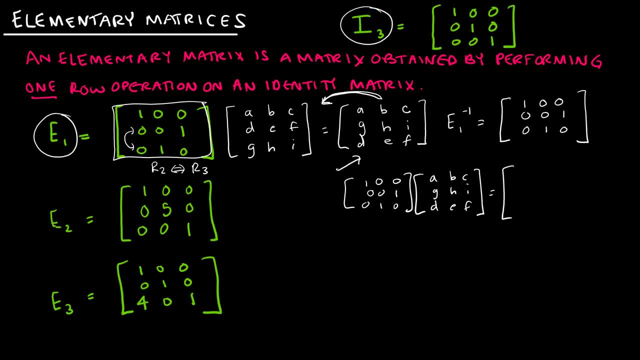 I shouldn't end up with a, b, c, d, e, f, g, h, i, And I in fact do So. the inverse again brings us back to where we started, So I'm going to erase this, because I don't have enough room to show everything. 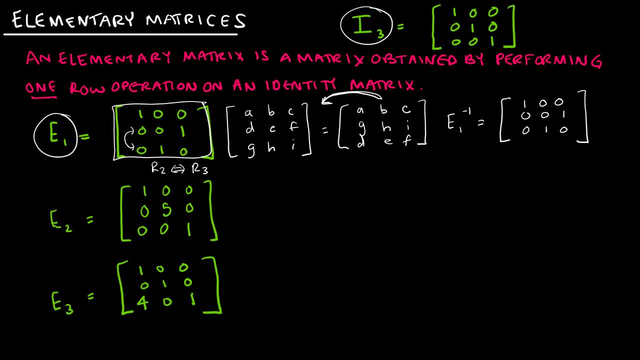 All right. So now let's take a look And again the row operation that would switch. it is, of course, just row 3 swapped with row 2. Or row 2 swapped with row 3.. Looking at E2, what would happen? 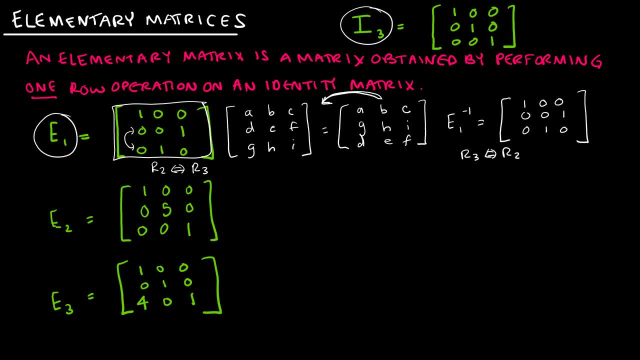 This one we should be familiar with, because this is very similar to our last example on the previous slide. This is obviously 5 times row 2 would be my new row 2.. Everything else remained the same. And again, notice, that's just one row operation. that's happening. 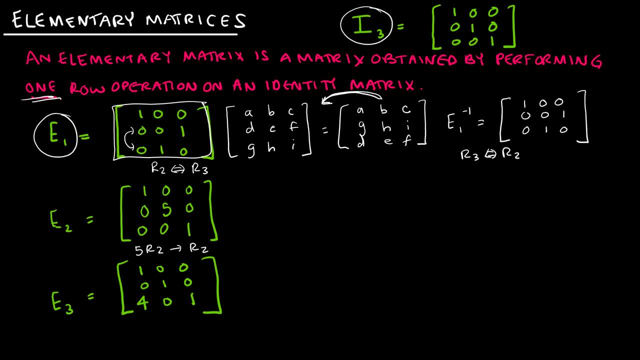 And I'm not going to multiply it by a, b, c, d, e, f, etc. We already know what's going to happen. We know that that second row is going to end up being 5,, 5, and 5.. 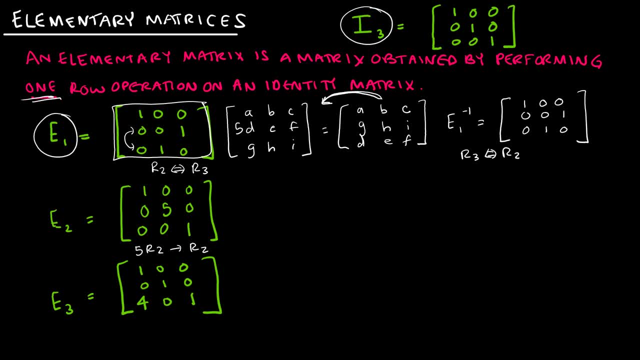 And hopefully you know that already, based on the example that we just did. So my question then is: what is E2 inverse? Which means what? would I have to take times my new matrix to get back to where I started? What would I have to do to undo what was done? 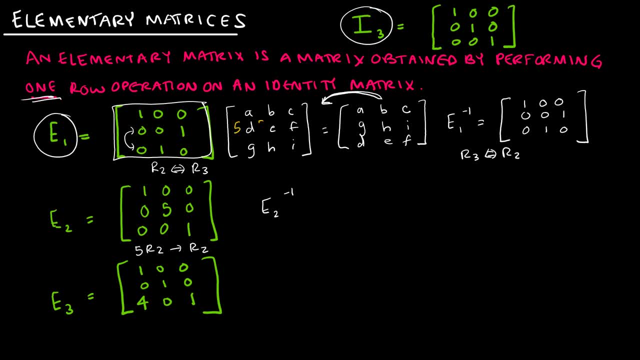 Well, if I had 5s here, then I would have to take 1, 0, 0, because I don't want anything in the first row to change, And 0, 0, 1, because I don't want anything in the last row to change. 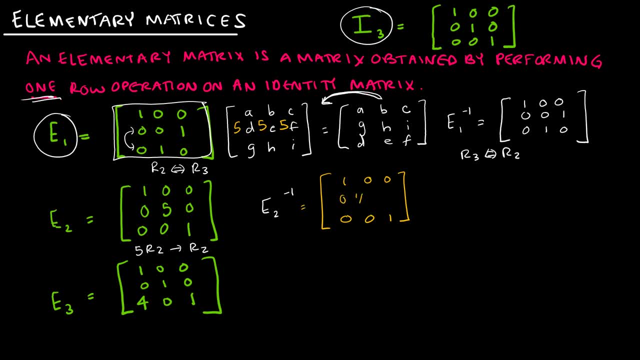 But my middle row. I want to be 1, 5th of what it was before And again, this correlates to my 1, 5th row 2 to be my new row 2.. Last one let's take a look at. 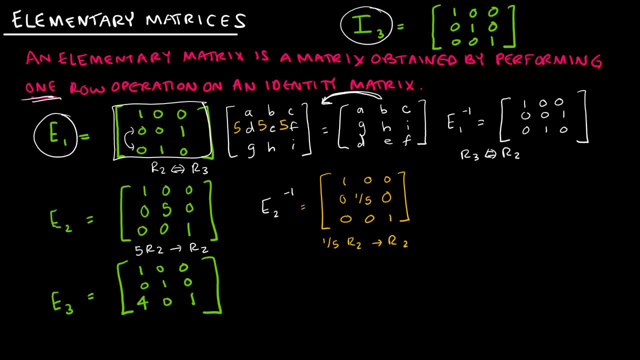 what the row operation would be. The first row remains the same. The second row remains the same. The third row: it looks like I took 4 times row 1 and added row 3 to be my new row 3.. 4 times row 1 plus row 3 to be my new row 3.. 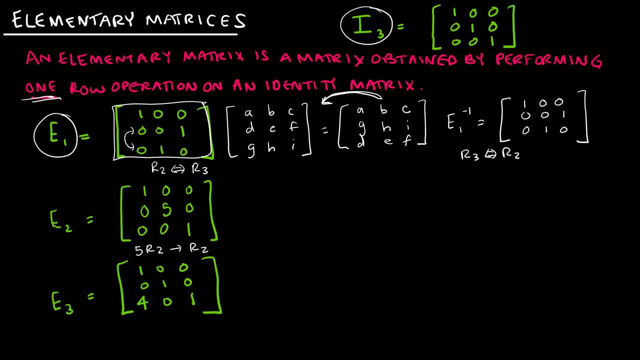 based on the example that we just did. So my question then is: what is E2 inverse? Which means? what? would I have to take times my new matrix to get back to where I started? What would I have to do to undo what was done? 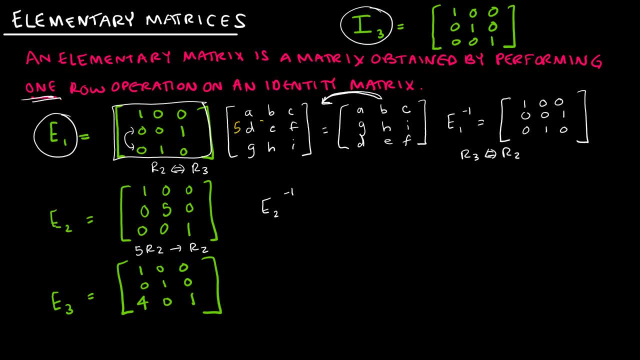 Well, if I had fives here, then I would have to take 1, 0, 0 because I don't want anything in the first row to change and 0, 0, 1 because I don't want anything in the last row to change. But my 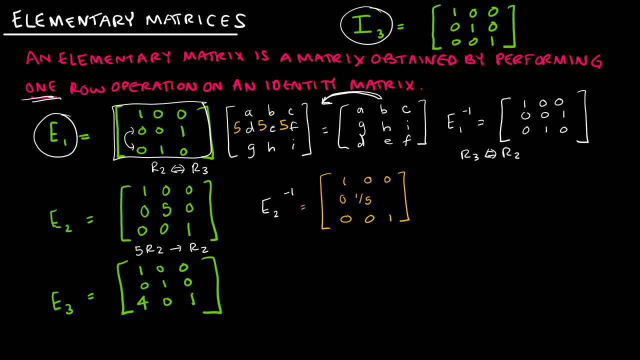 middle row. I want to be one-fifth of what it was before And again, this correlates to my one-fifth row 2, to be my new row 2.. Last one, let's take a look at what the row operation would be. The first row remains the 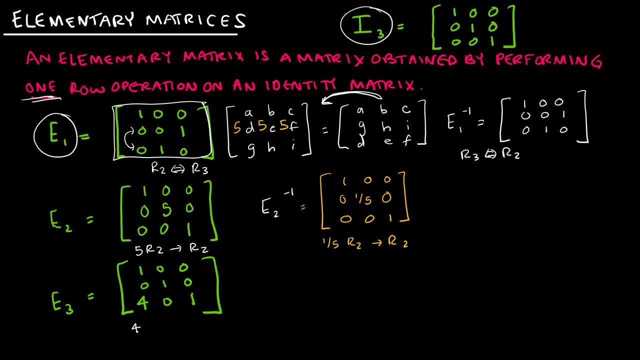 same. The second row remains the same. The third row: it looks like I took 4 times row 1 and added row 3 to be my new row 3.. 4 times row 1 plus row 3 to be my new row 3.. So now what? Now I have to. 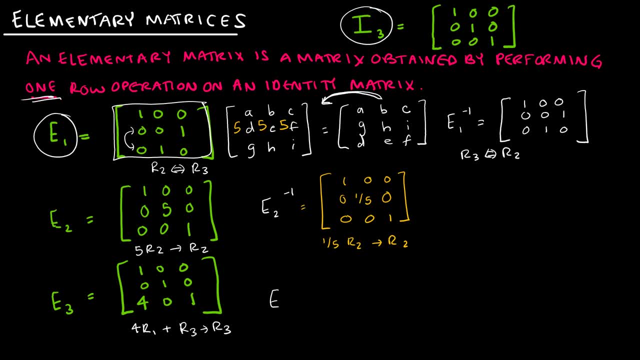 be able to undo that, And I can undo that by doing the same thing that I did in row 1.. I can undo that by going back and doing the same thing that I did in row 2.. And I can undo that by doing the same thing that I did in row 3.. 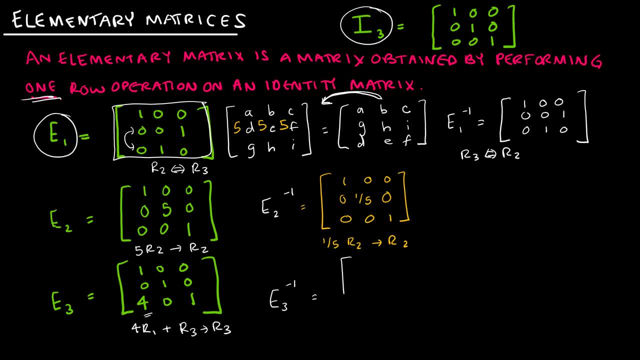 And that is the inverse of E3.. How can I undo what was done? So remember to undo what was done. I really want this guy to get back to 0, because that is going to get me back to what I started with, And so my row operation would be negative. 4, row 1 plus row 3 is my new row 3.. And then I have to undo that. 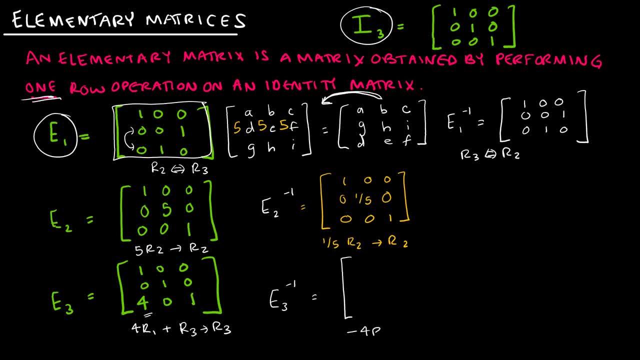 And then I have to undo that And that would look like 0, oops, 1, 0, 0, 0, 1, 0, negative: 4, 0, 1.. And that would be my inverse of E3.. 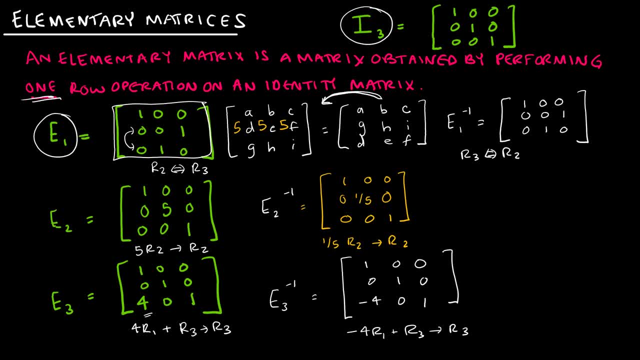 And again, I can always check that If I multiply E3 by the inverse of E3, and I'm not going to do that because I just don't have enough room- Okay, I lied, let's go ahead and do that. 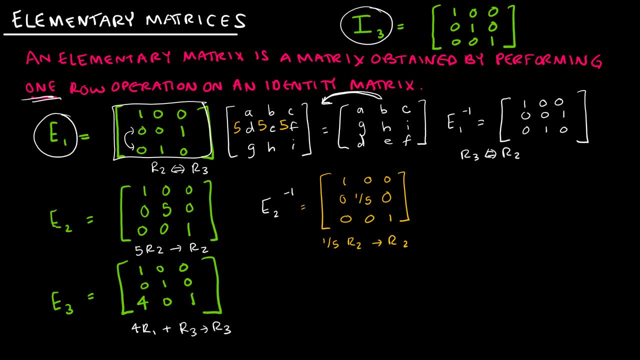 So now, what? Now I have to be able to undo that, Or what is the inverse of E3? How can I undo what was done? So, remember to undo what was done. I really want this guy to get back to 0, because that is going to get me back to what I started with. 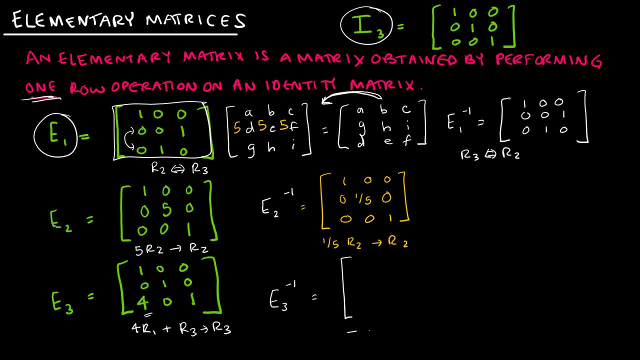 And so my row operation would be negative. 4 row 1 plus row 3 is my new row 3.. And that would look like 0, oops 1.. And that would look like 0, oops 1.. 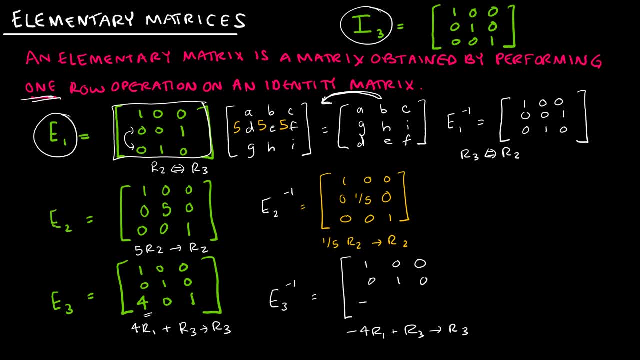 0, 0, 0, 1, 0, negative 4, 0, 1.. And that would be my inverse of E3.. And again, I can always check that If I multiply E3 by the inverse of E3, and I'm not going to do that because I just don't have enough room. 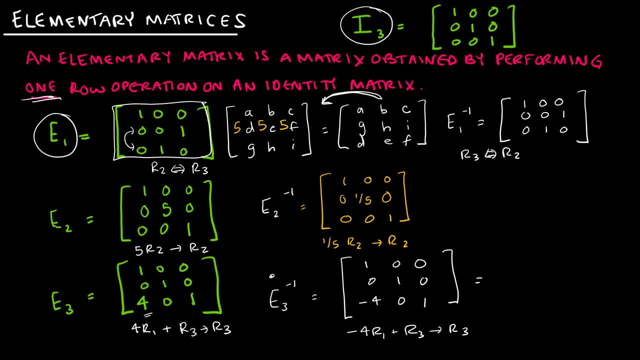 Okay, I lied, Let's go ahead and do that. If I multiply these, I'm going to get, hopefully, the identity matrix, because that's the whole point. So I get 1 plus 0 plus 0, and 0 plus 1 plus 0,- I'm sorry- 0 plus 0 plus 0, and 0 plus 0 plus 0.. 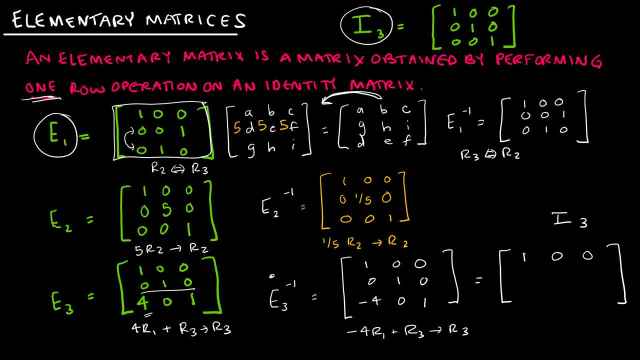 Next row, I'm going to get 0 plus 0 plus 0.. 0.. And then I'm going to get 0.. 0 plus 1 plus 0, and 0 plus 0 plus 0.. And then, my last row, I'm going to get 4 plus 0 plus negative 4, which is 0.. 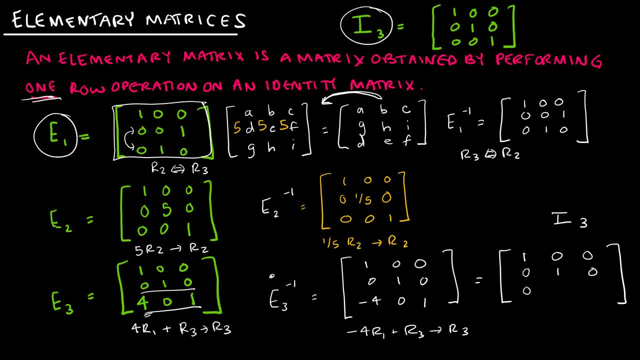 And then I'm going to get 0 plus 0 plus 0.. And then I'm going to get 0 plus 0 plus 1.. And notice, I did multiply the matrix by the inverse and I ended up back at the identity. 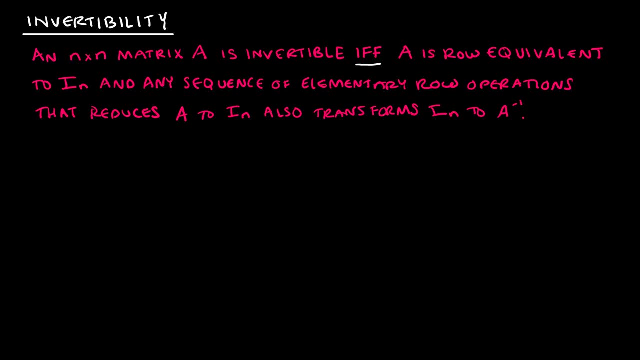 Now that we know what elementary matrices are, we would need to talk about invertibility. So we've talked about how to know if a 2 by 2 matrix is invertible, But, as we know in real life, when we're dealing with values that we can put into matrices, 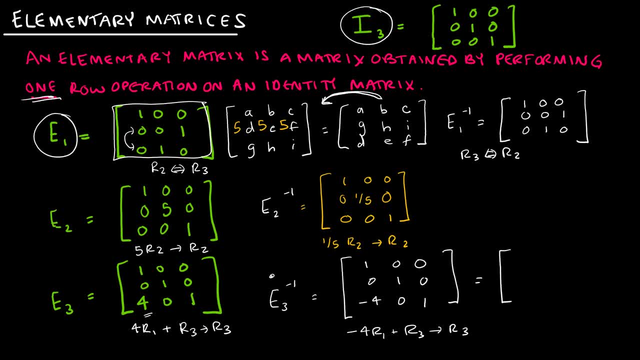 If I multiply these, I'm going to get, hopefully, the identity matrix, because that's the whole point. So I get 1 plus 0 plus 0, and 0 plus 1 plus 0,- I'm sorry, 0 plus 0 plus 0, and 0 plus 0 plus 0.. 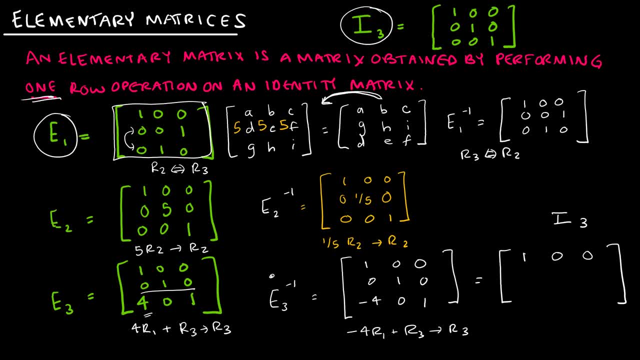 Next row, I'm going to get 0 plus 0 plus 0, and then I'm going to get 0 plus 1 plus 0, and 0 plus 0 plus 0.. And then, my last row, I'm going to get 4 plus 0 plus negative 4,, which is 0.. 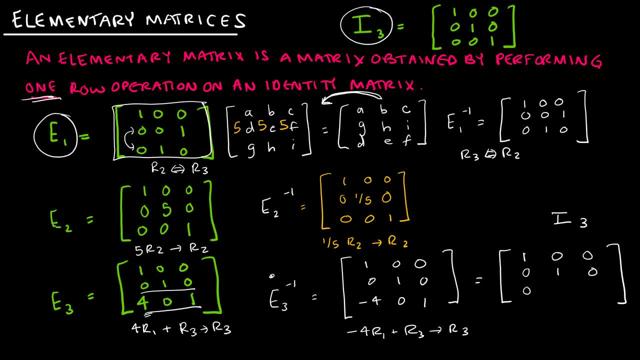 And then I'm going to get 0 plus 0 plus 0, and then I'm going to get 0 plus 0 plus 1.. And notice, I did multiply the matrix by the inverse and I ended up back at the identity. 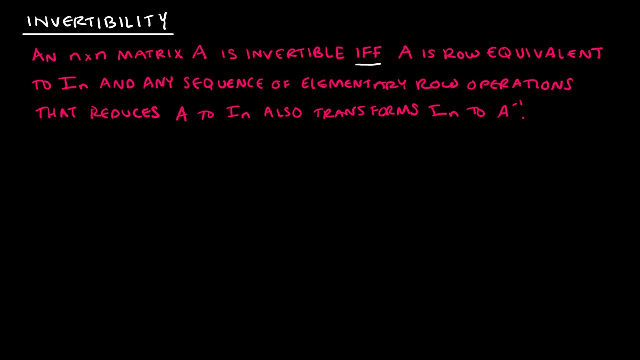 Now that we know what elementary matrices are, we would need to talk about invertibility. So we've talked about how to know if a 2 by 2 matrix is invertible, But, as we know in real life, when we're dealing with values that we can put into matrices, 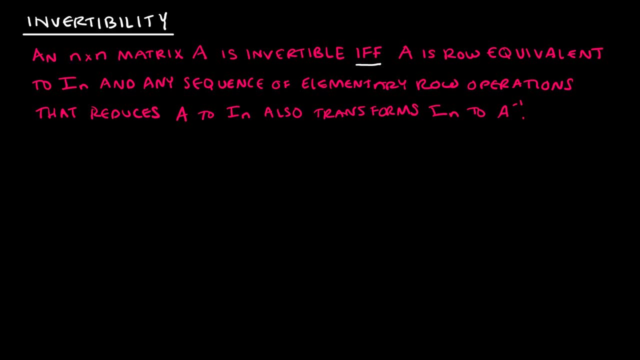 quite often it's not going to be 2 by 2.. So I'm going to try to point out- and this is going- We're going to be talking about this a lot. It's been a long time, so I apologize. 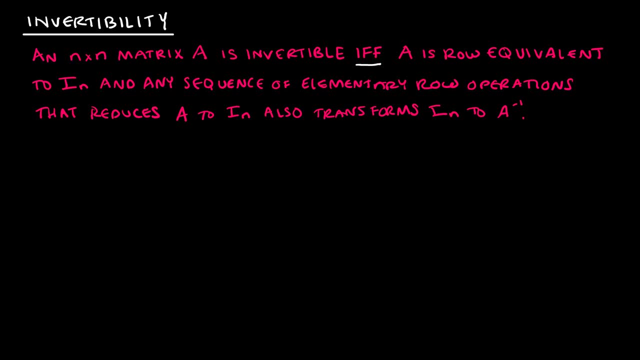 But I'm going to try to point out the important things as we go. First, it says an n by n matrix. So this is important because it tells us that this is a square matrix. If it's not a square matrix, it's not invertible. 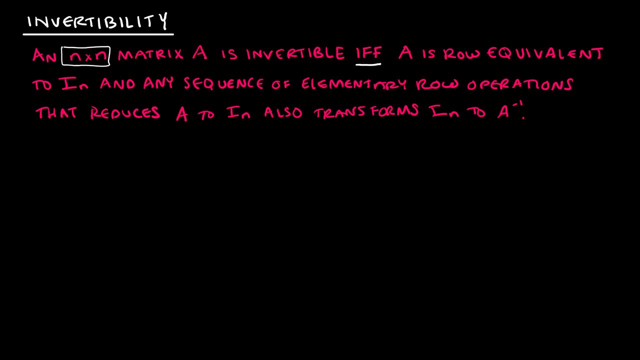 So it has to be a square matrix. It's invertible if and only if. So hopefully you've seen this notation before. If and only if means that we have to prove in 2. directions, Which means if p, then q needs to be proven. 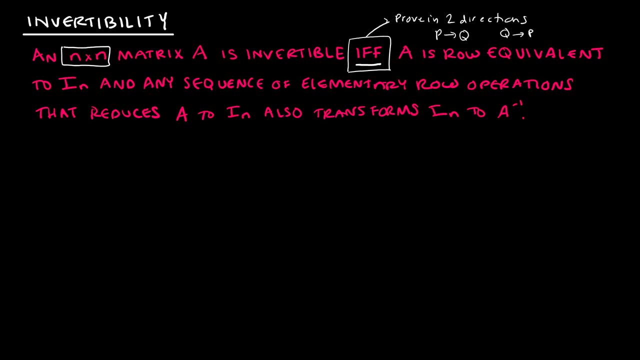 And if q, then p needs to be proven And we'll do that together. So hopefully I can make that make sense to you as we're proving this. So we're saying we have a square matrix. It's invertible if, and only if, a is row equivalent to i n. 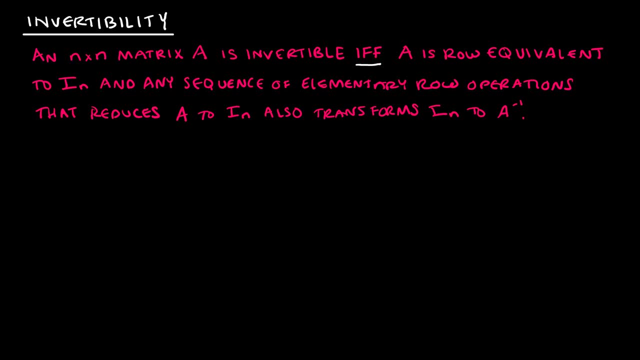 quite often it's not going to be 2 by 2.. So I'm going to try to point out- and we're going to be talking about this a long time, so I apologize, But I'm going to try to point out the important things as we go. 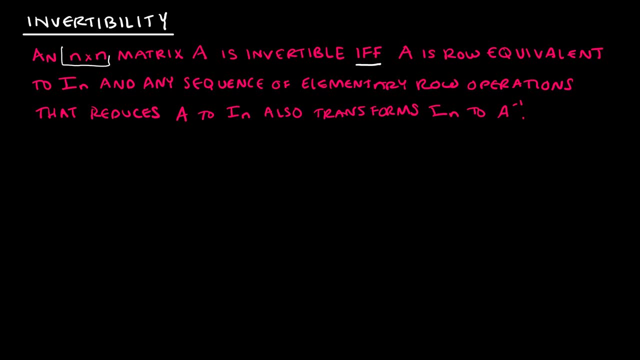 First, it says an n by n matrix. So this is important because it tells us that this is a square matrix. If it's not a square matrix, it's not invertible. So it has to be a square matrix. It's invertible if, and only if, 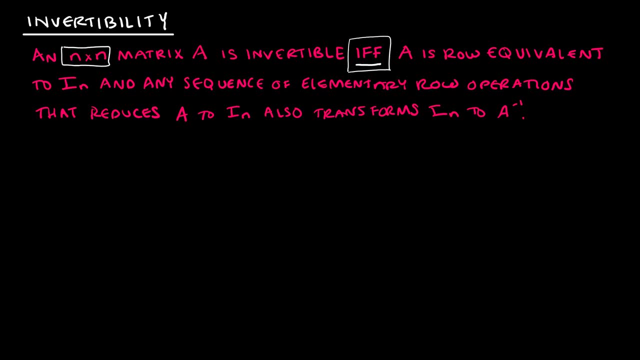 So hopefully you've seen this notation before. If, and only if, means that we have to prove in two directions, which means if p, then q, If q needs to be proven and if q then p needs to be proven, And we'll do that together. so hopefully I can make that make sense to you as we're proving this. 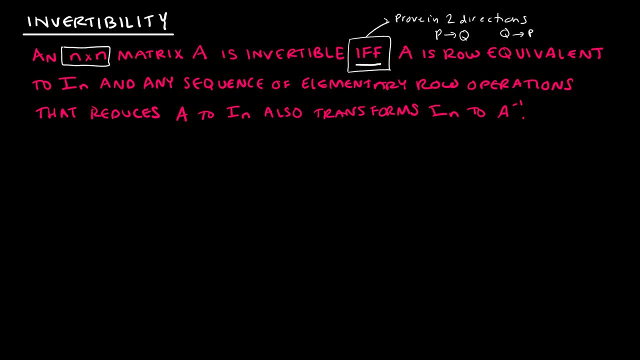 So we're saying we have a square matrix. It's invertible if, and only if, A is row equivalent to i n, which means, of course, to the identity matrix And any sequence of elementary row operations that reduces a to i n. 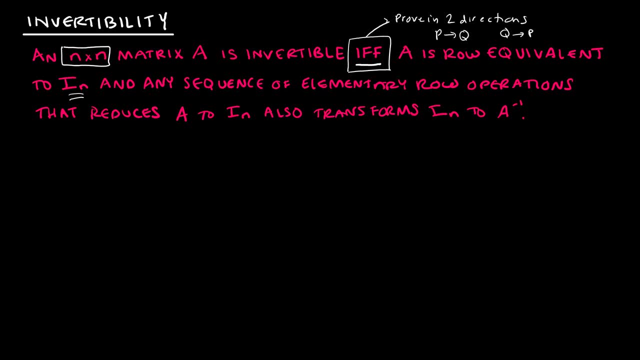 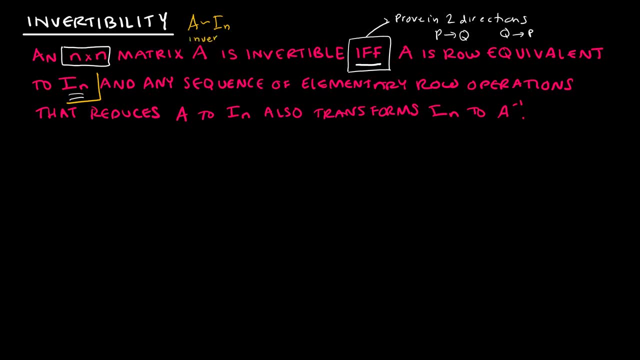 And then prove invertible. And then we need to assume it's invertible And prove that A reduces to the identity matrix. So that's what I'm talking about here when I talk about proving in two directions. So perhaps you've already done a lot of proofs like this. 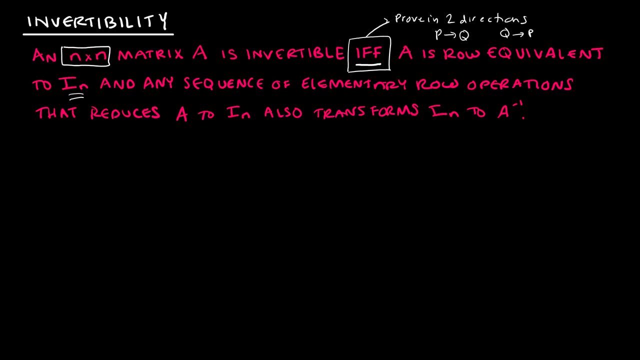 which means of course to the identity matrix, And any sequence of elementary row operations that reduces a to i n also transforms the identity to the inverse. So let's kind of focus here on the first part. An n by n matrix. a is invertible if, and only if, a is row equivalent to the identity matrix. 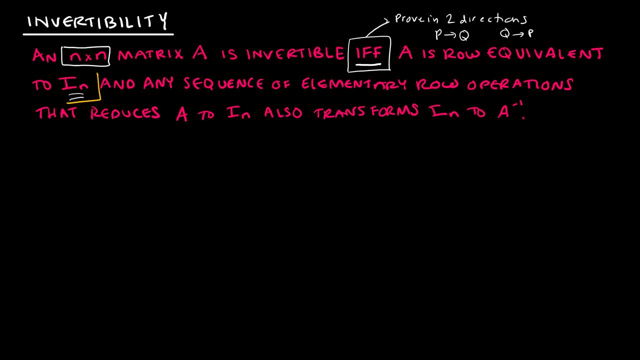 So, essentially, we need to assume that a will row reduce to the identity and then prove invertible, and then we need to assume it's invertible and prove that a reduces to the identity matrix. So that's what I'm talking about here when I talk about proving in two directions. 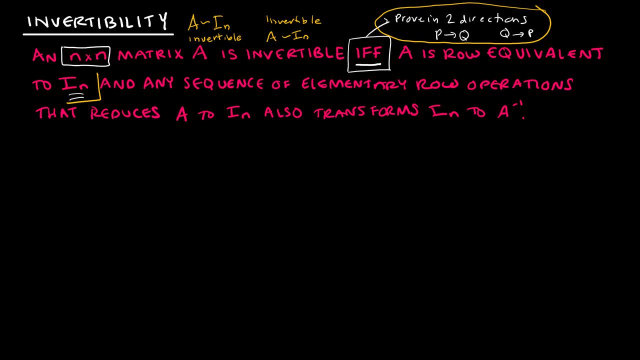 So perhaps you've already done a lot of proofs like this, But in case you haven't, that's what it means when we say if, and only if, We'll get to all of this stuff here once we've done the proof. So the first direction- and I wasn't going to try to write and talk at the same time- 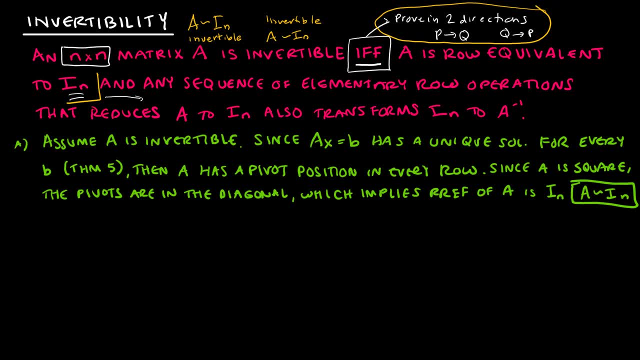 So here's the first direction. So I'm assuming a is invertible. That's this guy. So I'm going to assume a is invertible. Since ax equals b has a unique solution for every b, and that's theorem 5 from your textbook. 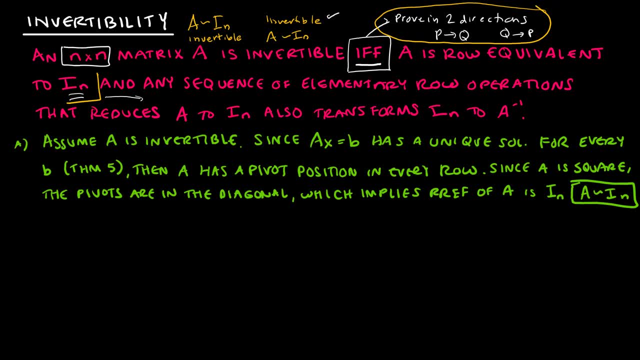 then a has a pivot position in every row, which we already know from- I don't remember what theorem it was, but in our last chapter. Since a is a square matrix, the pivots are in the diagonal, which we know. that implies that reduced row echelon form of a is the identity matrix. 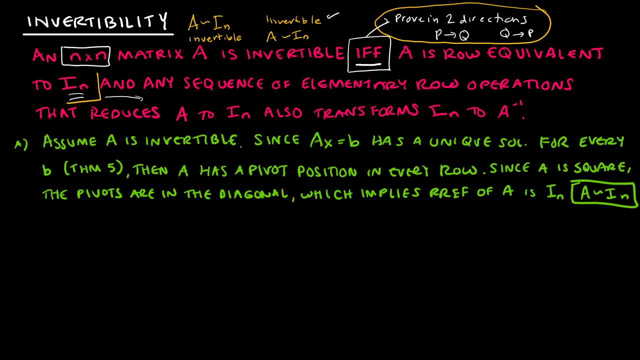 So let's take a look at that again. We assume it's invertible, We know it has a solution For every b, then a has a pivot position in every row And again we've got a square matrix and the pivot position in every row means these are all going to be ones. 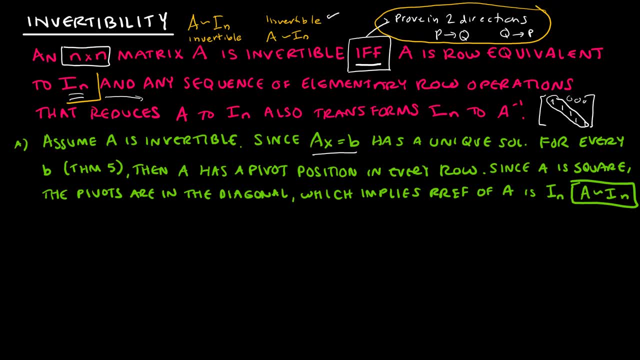 however many ones we need, and everything else is going to be zeros, because that's how it works. And no, I'm sure I didn't get all of the zeros in here correctly, but you get the idea. I think I'm missing several zeros. 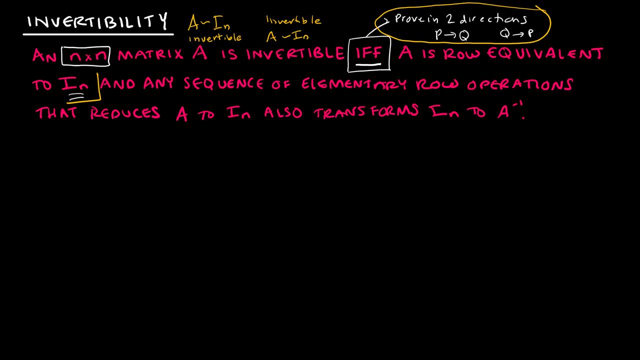 But in case you haven't, that's what it means when we say if, and only if, We'll get to all of this stuff. We'll get to all of this stuff Here once we've done the proof. So the first direction: 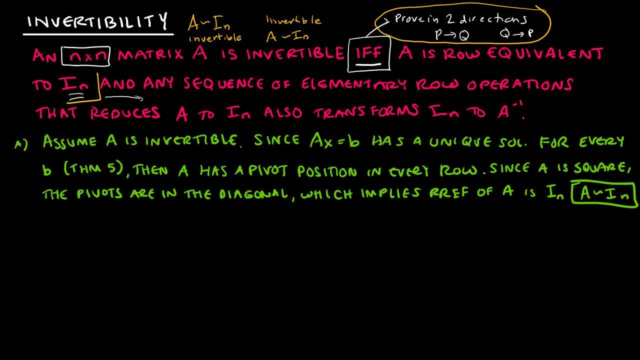 And I wasn't going to try to write and talk at the same time. So here's the first direction. So I'm assuming A is invertible. That's this guy. So I'm going to assume A is invertible. Since AX equals B, has a unique solution for every B. 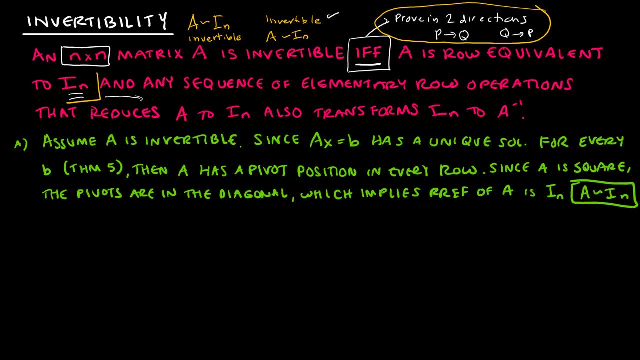 And that's theorem 5 from your textbook. Then A has a pivot position in every row, Which we already know from the previous example- I don't remember what theorem it was, but in our last chapter, Since A is a square matrix, the pivots are in the diagonal, which we know that implies 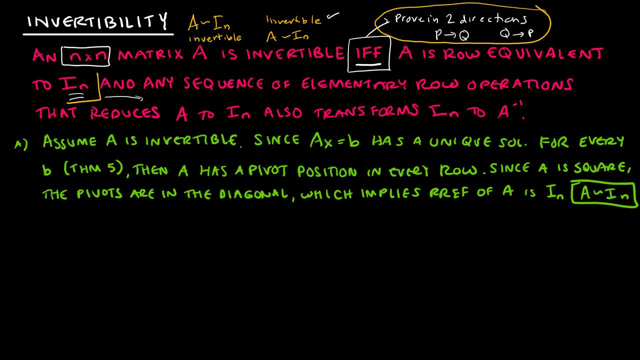 that reduced row echelon form of A is the identity matrix. So let's take a look at that again. We assume it's invertible. We know it has a solution for every B. Then A has a pivot position in every row And again we've got a square matrix. 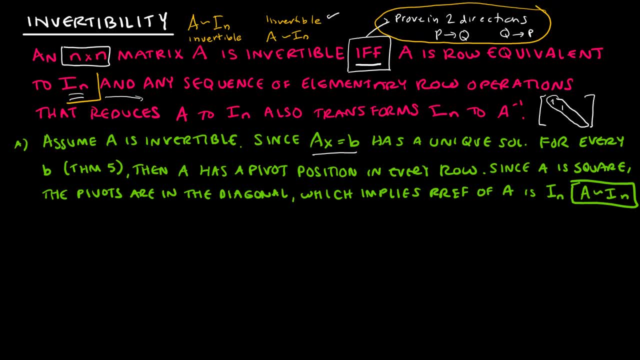 And the pivot position in every row means these are all going to be 1s, however many 1s we need, And everything else is going to be 0s, because that's how it works, And no, I'm sure I didn't get all of the 0s in here correctly. 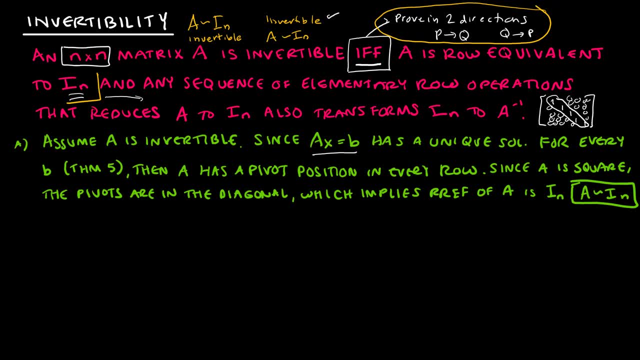 But you get the idea- I think I'm missing several 0s- But you get the idea that we know that if we have a matrix that is a square matrix and the only values are the diagonal and they're all 1s. 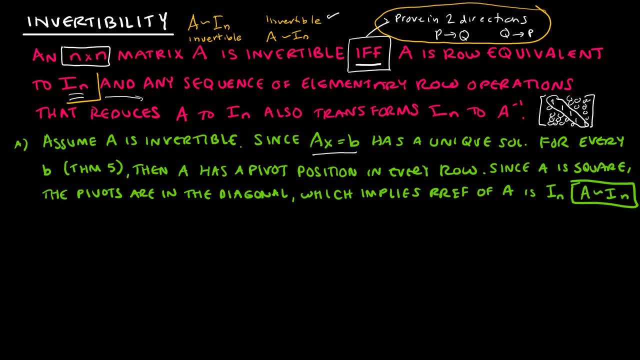 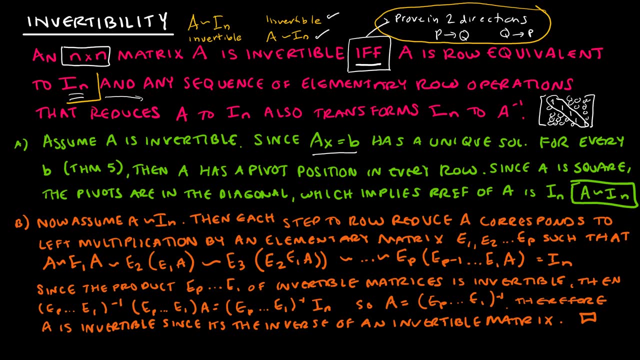 then it, of course, is the identity matrix. So we've proven the first direction. Now let's prove the second direction, which is, as you can see, a little bit more involved. So I'm going to try to walk you through this. 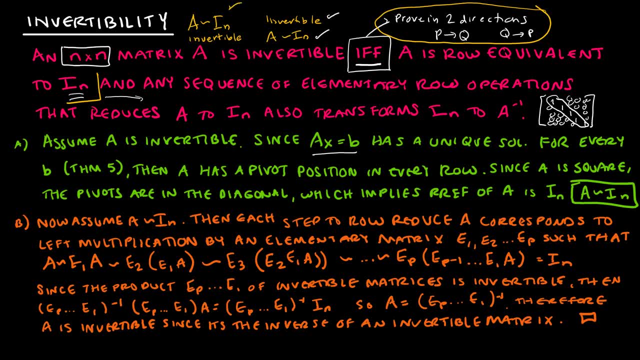 We are going to assume now that A row reduces to the identity. That means that each step to row reduce A corresponds to the identity. So we're going to assume that A row reduces to the identity And that corresponds to left multiplication by an elementary matrix. 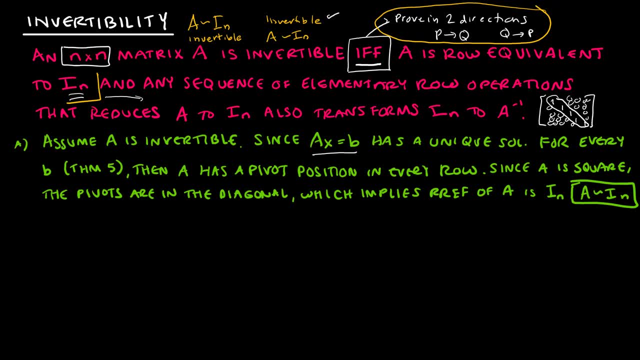 But you get the idea That we know that if we have a matrix that is a square matrix and the only values are the diagonal and they're all ones, then it of course is the identity matrix. So we've proven the first direction. 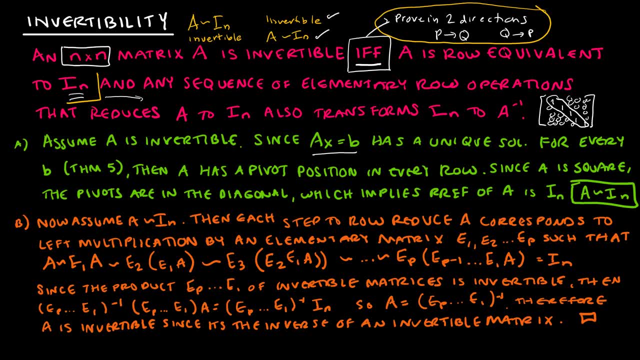 Now let's prove the second direction, which is, as you can see, a little bit more involved. So I'm going to try to walk you through this. We are going to assume now that a row reduces to the identity. That means that each step to row reduce a corresponds to left multiplication by an elementary matrix. 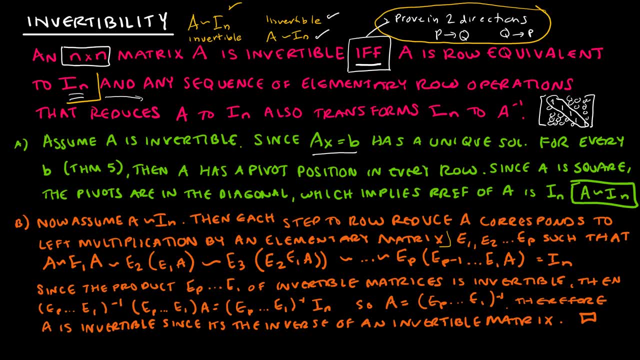 So let's talk about this sentence. We just, on our last slide, talked about left multiplication and what that did. That's what we're talking about here. So we're saying we can do all of these row reduction steps using matrices instead of row operations. 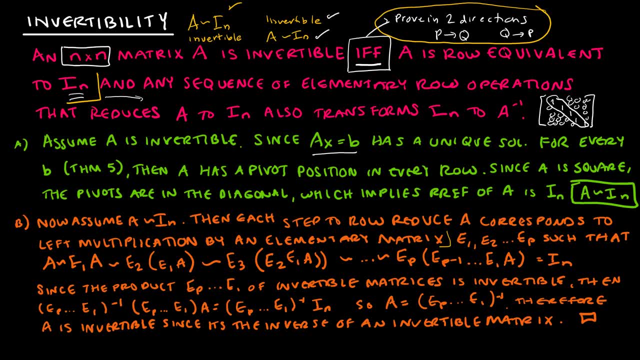 and we're going to continue to multiply on the left side, because that's the side we're going to need to multiply on for this all to work out. And so, essentially, what's going to happen is, if I have an elementary row, operation 1,, 2,, 3, all the way up to P. 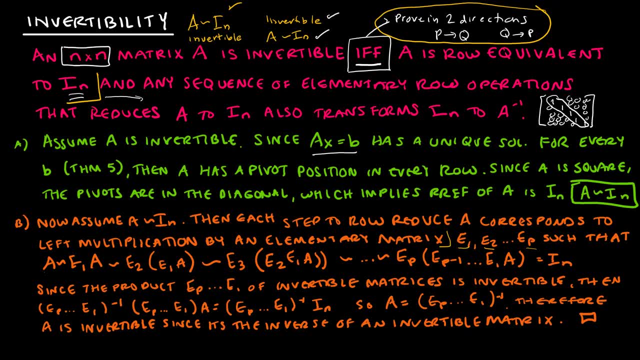 then I would start with the first. So I'm going to have A and then I'm going to do. that's equivalent to the elementary row operation: the first one times A, and then the second one times The result, and then the third one times the result, et cetera. 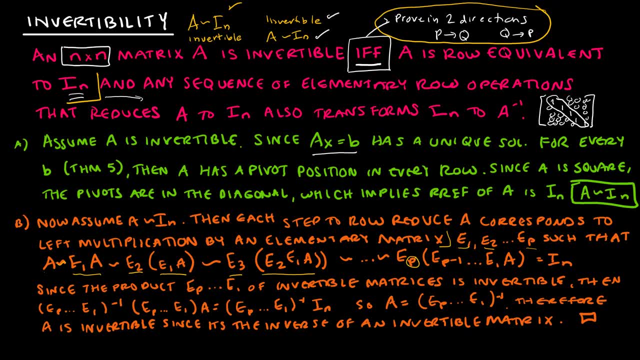 And we would continue to do that up until the point where we have this very last row operation And when I'm done, I'm going to end up with the identity matrix, because that's what we're assuming here, that A does row reduce to the identity matrix. 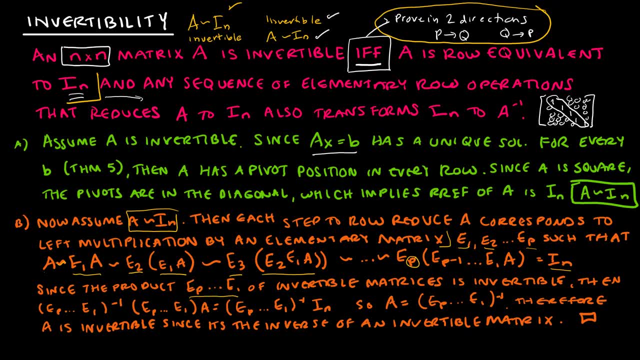 Now, since the product of all of those elementary row operations of invertible matrices is the number of rows, then the number of rows is the number of rows. So if A is invertible, then we can say that if I take the inverse times, all of those row operations times A. 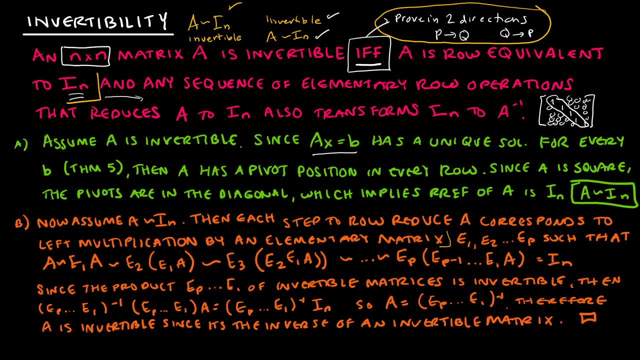 So let's talk about this sentence. We just, on our last slide, talked about left multiplication and what that did. That's what we're talking about here. So we're saying we can do all of these row reduction steps using matrices instead of row operations. 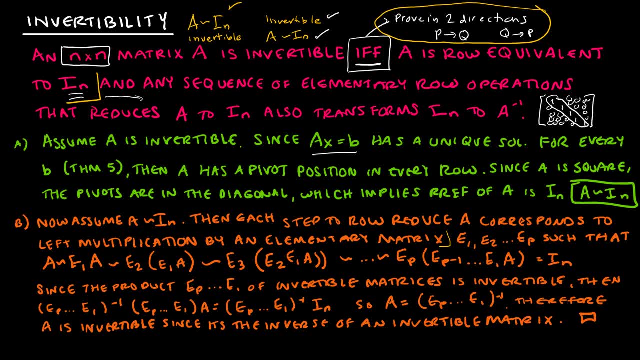 And we're going to continue to multiply on the left side, because that's the side we're going to need. So we're going to continue to multiply on the left side and then we're going to continue to multiply on for this all to work out. 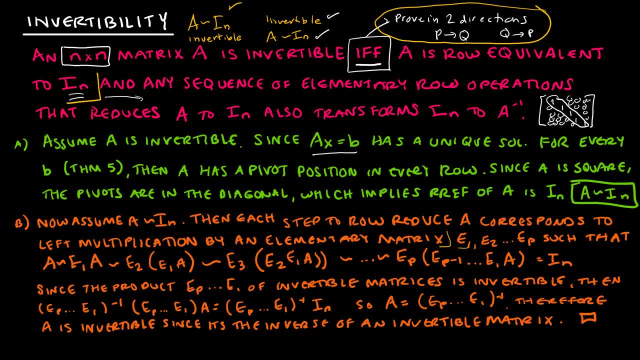 And so essentially what's going to happen is if I have an elementary row operation- 1,, 2,, 3, all the way up to P- then I would start with the first. So I'm going to have A and then I'm going to do that's equivalent to the elementary row operation. 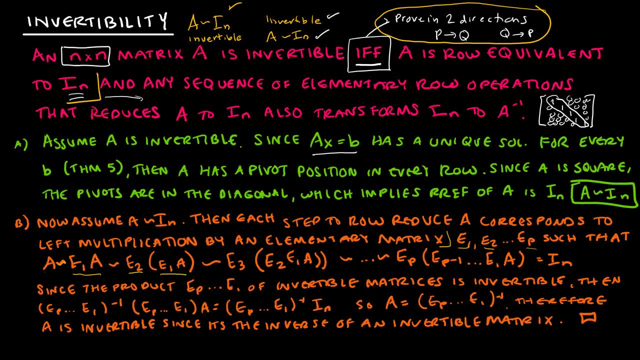 the first one times A, and then the second one times the result, and then the third one times the result, etc. And we would continue to do that up until the point where we have this result. So we're going to continue to multiply on this very last row operation. 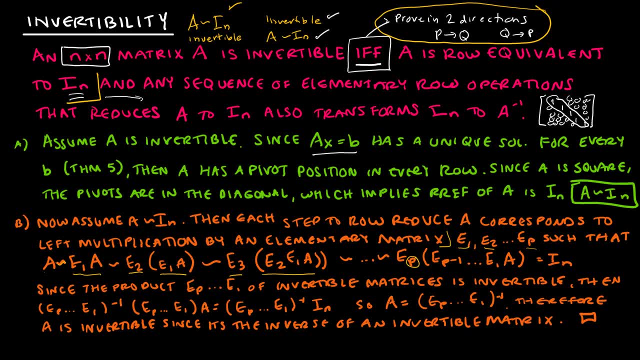 And when I'm done, I'm going to end up with the identity matrix, because that's what we're assuming here, that A does row reduce to the identity matrix? Now, since the product of all of those elementary row operations of invertible matrices is invertible, 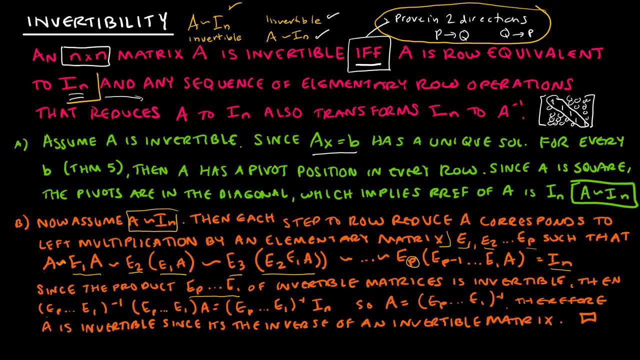 then we can say that if I take the, the inverse times all of those row operations times A, then that's going to be equivalent to the inverse of all of those operations times the identity. So why is that true? Because all I did was left multiplication. 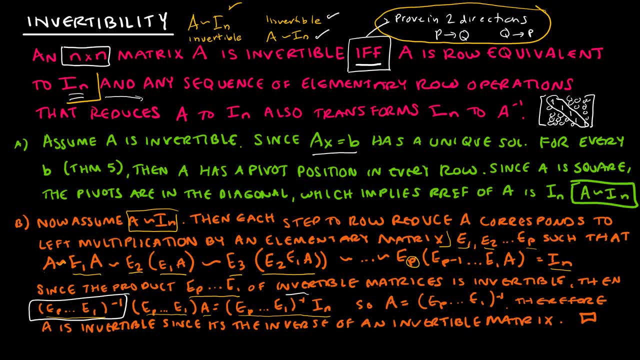 times the identity. So what I'm going to do is I'm going to take the inverse times, the inverse on each side from what I had just shown here. Now, that also means, then that A, because, as you'll notice what's going to happen with those two? 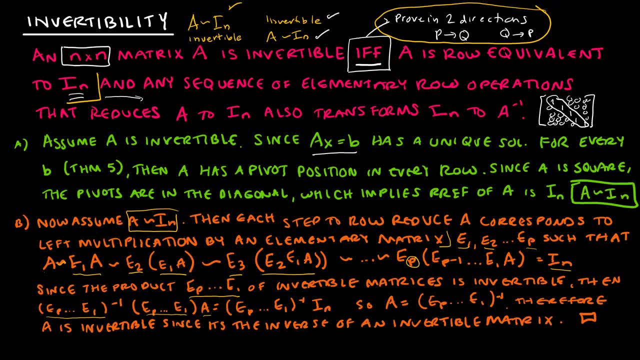 then that's going to be equivalent to the inverse of all of those operations times the identity. So why is that true? Because all I did was left multiplication times the inverse on each side from what I had just shown here. Now that also means then that A, because, as you'll notice, what's going to happen with those two? 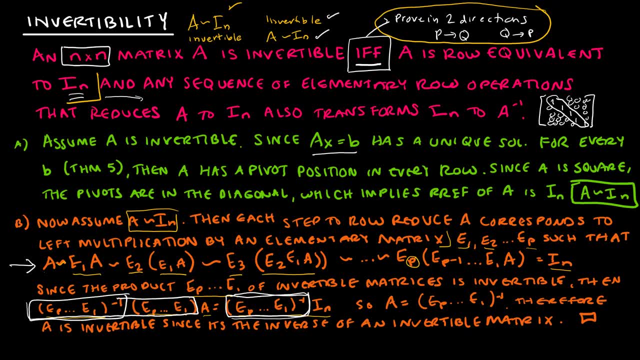 So A is equivalent to the inverse of all of that, So A is equivalent to the inverse of all of those operations times the identity. Therefore, A is invertible, since it's the inverse of an invertible matrix. So now we've proven the other direction. 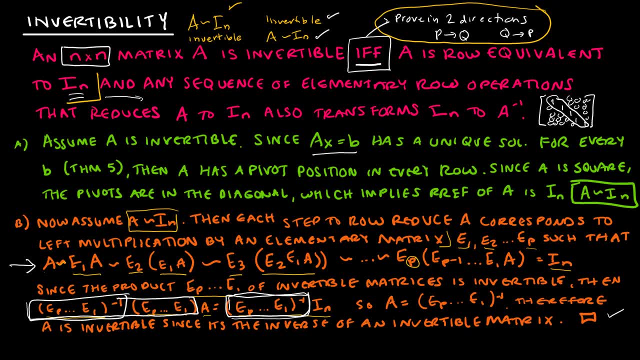 So, essentially, I'm done with the proof, But we really haven't gotten to why this is so important. and it is so important and awesome And it's what we're going to do: moving forward for anything that's not a 2x2 matrix. 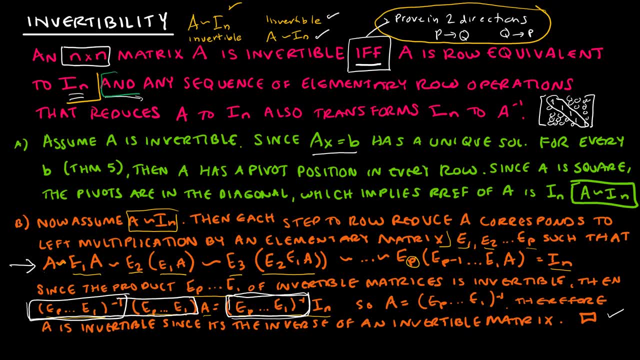 So let's go back to this, And any sequence of elementary row operations that reduces A to the identity also transforms the identity to the inverse. So here's essentially what that means. So we have any sequence of elementary row operations, So I'm going to do the row operations, all of these guys, and that's what this is saying here. 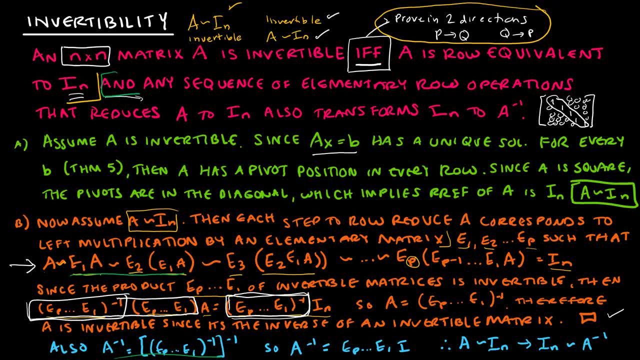 All of these row operations that reduces a to the identity will also take the identity and turn it into the inverse of a, which is fantastic. So why do I care about that? Why am I so excited? I'm math geeking out about it. 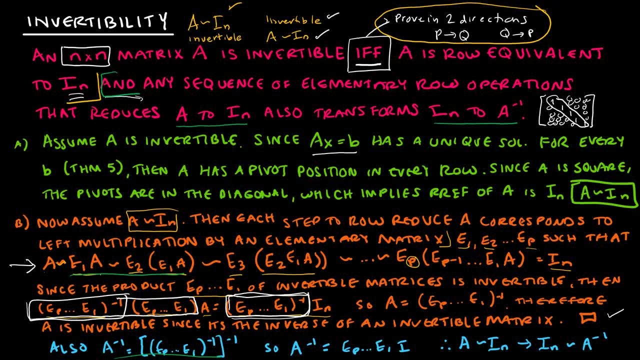 Because all I have to do is do my normal row operations to reduce a to the identity, and when I do that simultaneously, I'm going to be turning the identity into the inverse, and so that is how I'm going to solve for the inverse, and that's what all of this stuff. 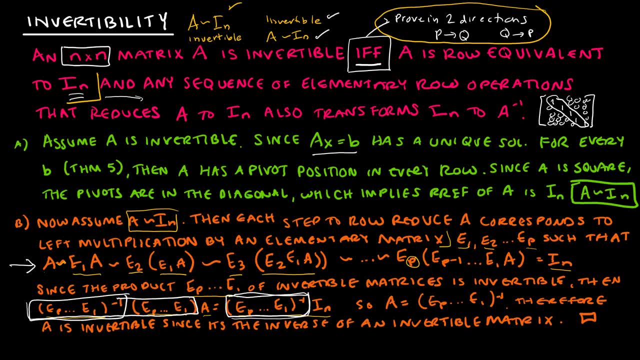 So A is equivalent to the inverse of all of that times the identity. Therefore A is invertible, since it's the inverse of an invertible matrix. So now we've proven the other direction. So essentially I'm done with the proof. 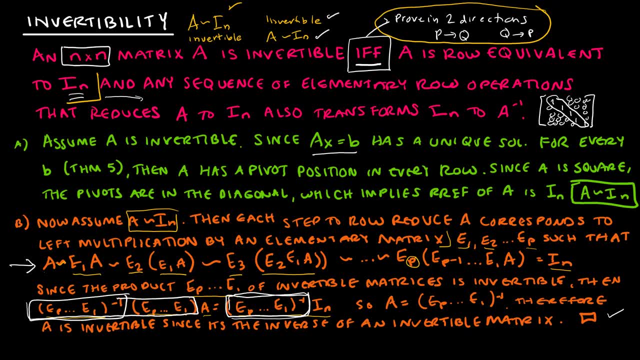 But we really haven't gotten to why this is so important. And it is so important and awesome And it's what we're going to do, moving forward for anything that's not a two by two matrix. So let's go back to this. 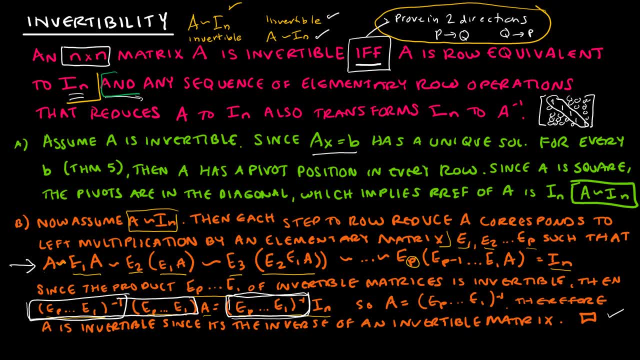 And any sequence of elementary row operations that result in an invertible matrix that reduces A to the identity also transforms the identity to the inverse. So here's essentially what that means. So we have any sequence of elementary row operations, So I'm going to do the row operations. 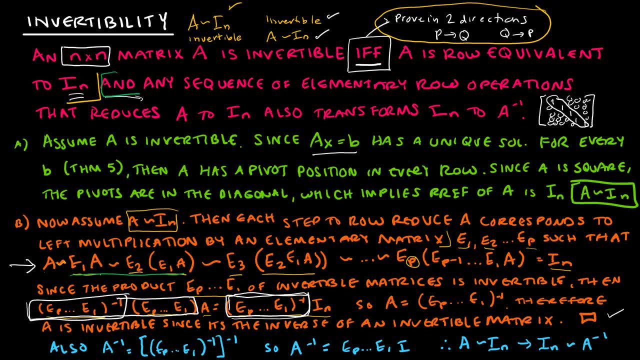 all of these guys- and that's what this is saying here- All of these row operations that reduces A to the identity will also transform the identity to the inverse, So I can also take the identity and turn it into the inverse of A, which is fantastic. 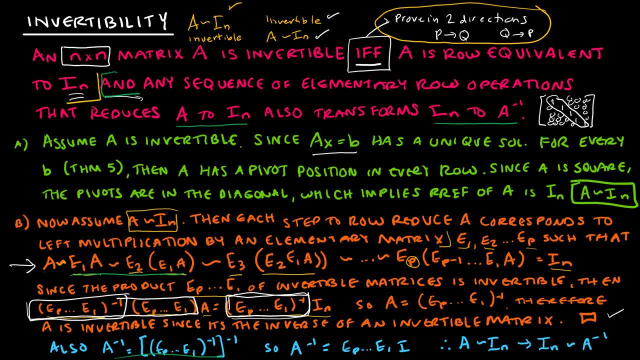 So why do I care about that? Why am I so excited? I'm math geeking out about it, Because all I have to do is do my normal row operations to reduce A to the identity, And when I do that simultaneously, I'm going to be turning the identity. 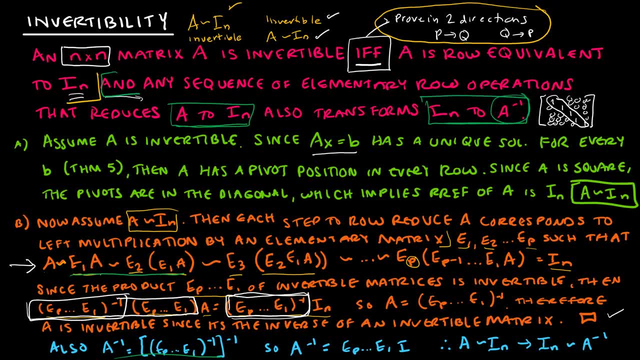 into the inverse, And so that is how I'm going to solve for the inverse, And that's what all of this stuff down here means. So that might be very confusing. I tried to explain it as best I could, but it really makes so much more sense. 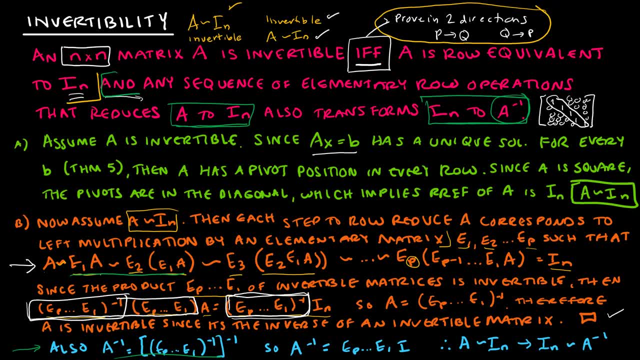 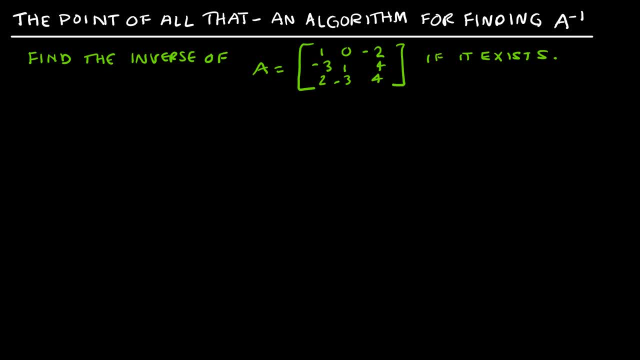 when we actually do a question together using this. That brings us to the point of everything that we have just proven, which is the algorithm for finding A inverse. So, in case you fell asleep while I was doing that last proof, which is possible, 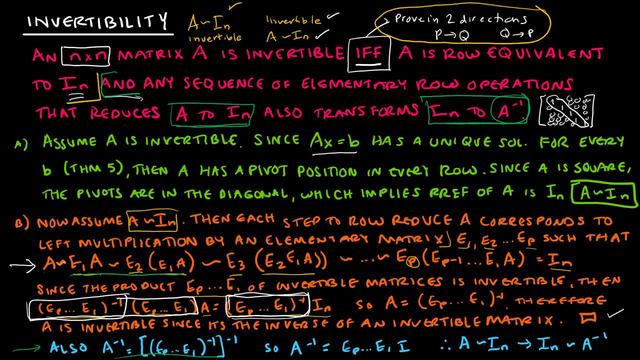 down here means. So that might be very confusing. I tried to explain it as best I could, but it really makes so much more sense when we actually do a question together using this. That brings us to the point of everything that we have just proven. 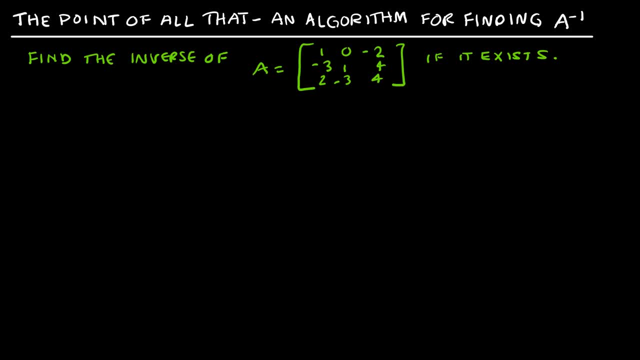 which is the algorithm for finding a inverse. So in case you fell asleep while I was doing that last proof, which is possible, let's just recap what we know. We know that if I can take a and row, reduce it to the identity matrix, then, at the very same time, the identity matrix, using those 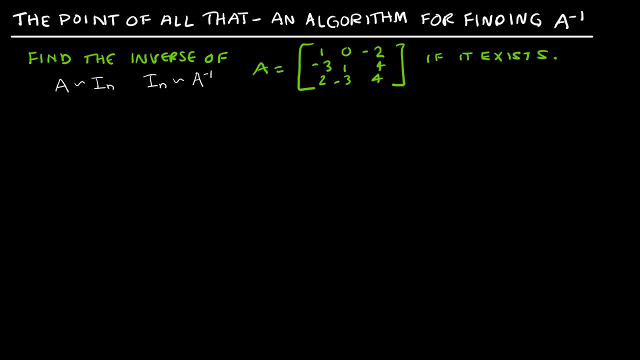 same row, operations can become a inverse, or will become a inverse if it exists, of course. So this is how we know. if it exists, says is we do the math. So what that means for us is that we're going to take A 1, 0,. 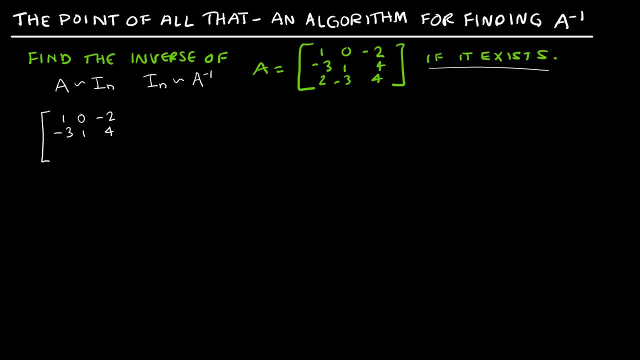 negative 2, negative 3, 1, 4, 2, negative 3, 4 on the left side. On the right side we're going to put the identity matrix. So what I'm going to do is I'm just going to do my normal row operations to turn the left side into the border and then got the A- 3,5,2,0,2,2 and then theN that-и-3,4 On the left side. on the right side we're going to put the identity matrix. So what I'm going to do is I'm just going to do my normal row operations to turn the left side into theators, to turn the right side into the指r, to ner. 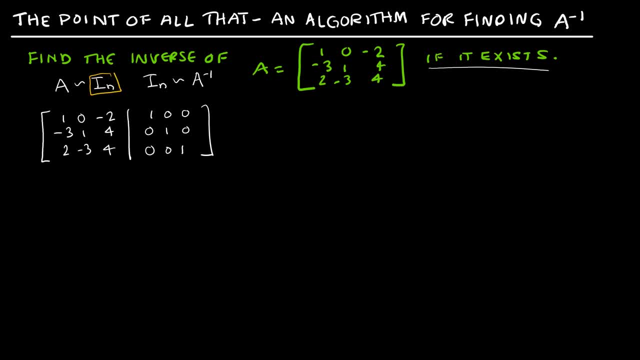 side into reduced row echelon form, also known as the identity matrix in this case, because that's what's going to happen on the left. So as I'm doing that, I also have to do those same row operations on the right side, and when I get done, I'm just magically going to have a inverse. 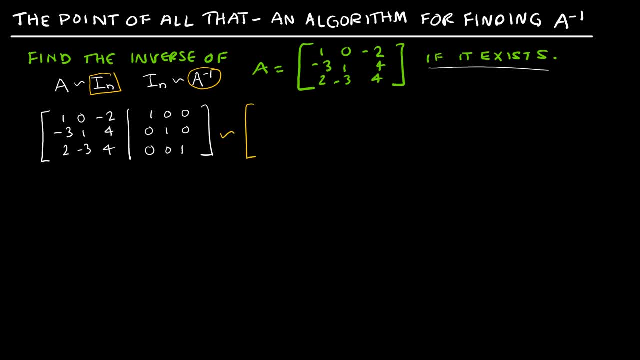 So let's do this. I should have done it ahead of time, but I didn't, so I'm hoping I don't mess up. So the first thing I'm going to do is, of course, I have 1 as my pivot, which is what I wanted. 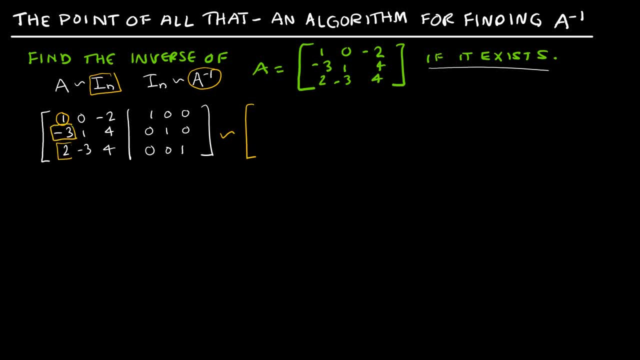 I need negative 3 to turn into a 0 and 2 to turn into a 0.. So my first row operation- I'm going to go ahead and copy this- My first row operation is going to be to take 3 times row 1 and add it to row 2.. So 3 times 1 is 3, plus negative 3 is 0.. 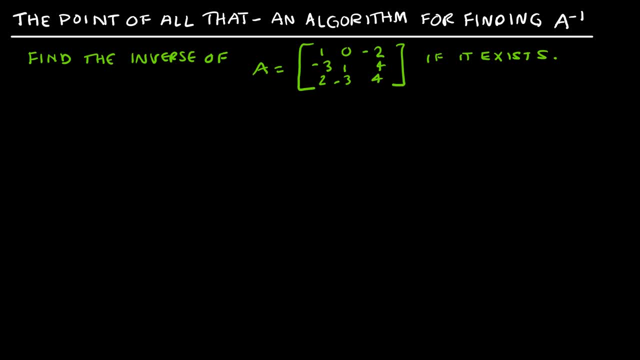 let's just recap what we know. We know that if I can take A and row, reduce it to the identity matrix, then at the very same time, the identity matrix using those same row operations can become A inverse, or will become A inverse If it exists, of course. 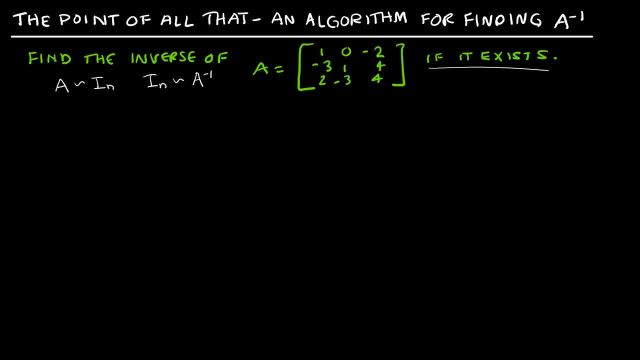 So this is how we know if it exists is we do the math. So what that means for us is that we are going to take A A 1, 0, negative 2, negative 3, 1, 4, 2, negative 3, 4, on the left side. 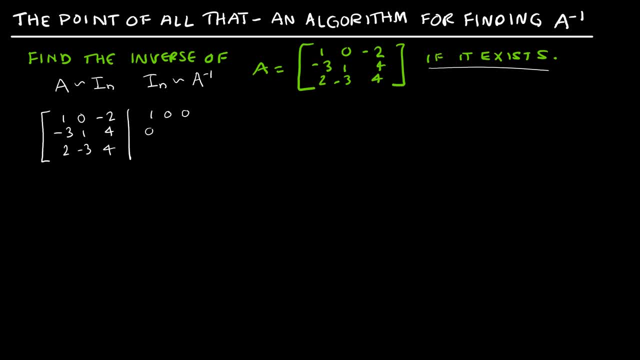 On the right side we're going to put the identity matrix. So what I'm going to do is I'm just going to do my normal row operations to turn the left side into reduced row echelon form, also known as the identity matrix in this case. 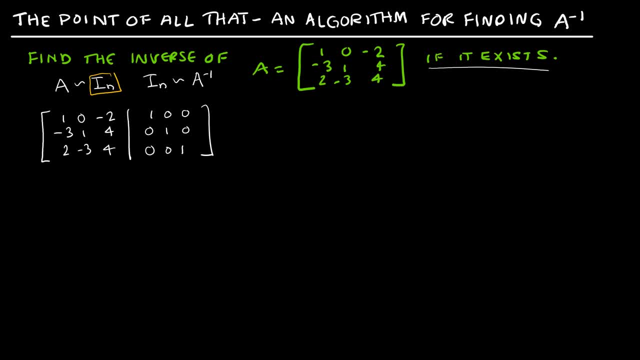 because that's what's going to happen on the left. So as I'm doing that, I also have to do those same row operations on the right side, and when I get done, I'm just magically going to have a inverse. So let's do this. 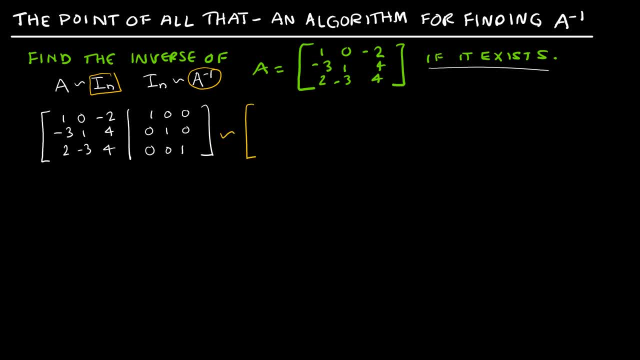 I should have done it ahead of time, but I didn't, so I'm hoping I don't mess up. The first thing I'm going to do is, of course, I have 1 as my pivot, which is what I wanted. 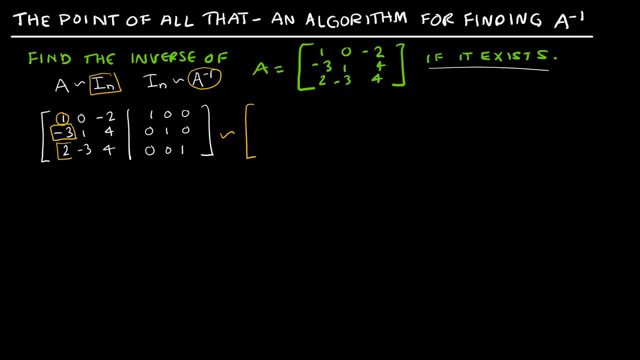 I need negative 3 to turn into a 0 and 2 to turn into a 0.. So my first row operation- I'm going to go ahead and copy this- My first row operation is going to be to take 3 times row 1 and add it to row 2.. 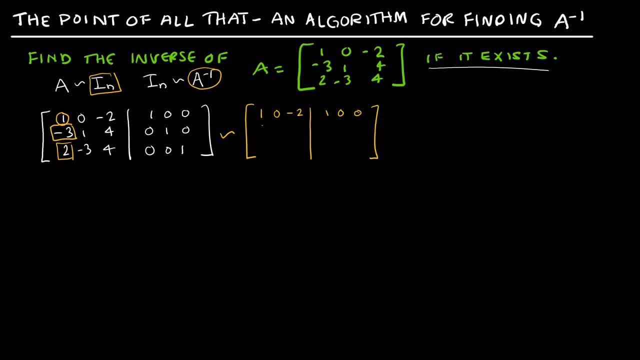 So 3 times 1 is 3, plus negative 3 is 0.. 0 plus 1 is 1.. Negative: 6 plus 4 is negative. 2. 3 plus 0 is 3.. 0 plus 1 is 1, and 0 plus 0 is 0.. 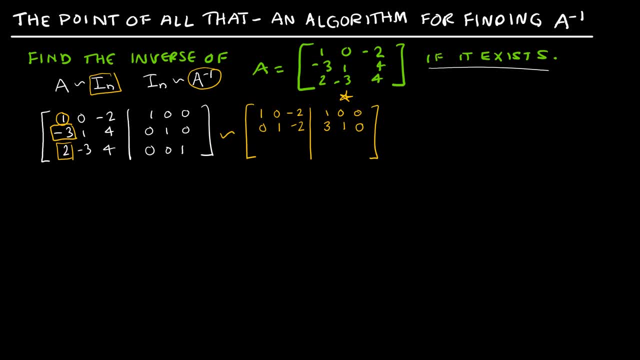 So again, here's the first row. So I'm going to do this. I'm going to do this. Here's just your reminder. Whatever row operation you're doing to the left side, you continue it on the right side. Then I also need to take row 1 times negative 2 and add it to row 3.. 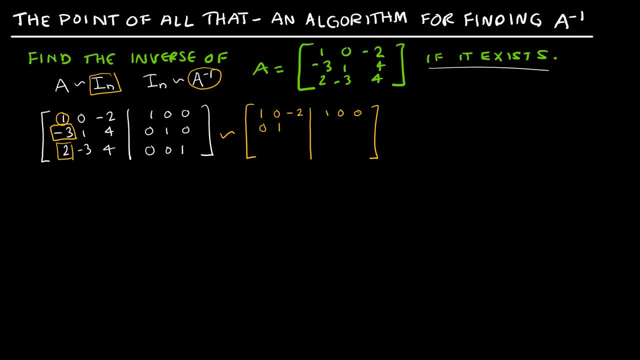 0 plus 1 is 0.. 1 is 1. Negative. 6 plus 4 is negative, 2.. 3 plus 0 is 3.. 0 plus 1 is 1, and 0 plus 0 is 0.. 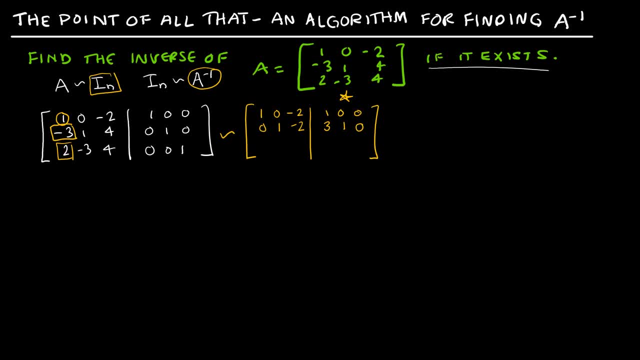 So again, here's just your reminder: whatever row operation you're doing to the left side, you continue it on the right side. Then I also need to take row 1 times negative 2 and add it to row 3.. So negative 2 plus 2 is 0.. Negative 2 times 0 is 0, plus negative 3.. 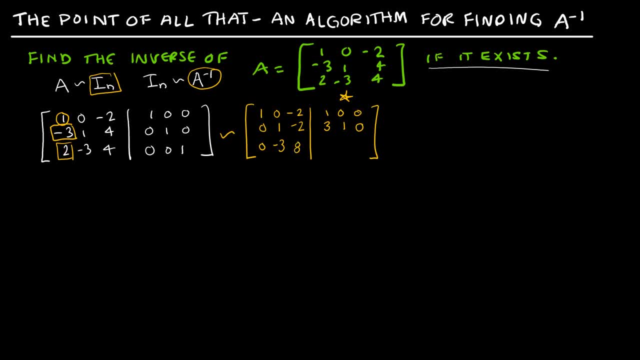 Positive: 4 plus 4 is 8.. Negative: 2 plus 0 is negative, 2. 0 plus 0 is 0, and 0 plus 1 is 1.. So far, so good. I have a pivot right here and I've got a pivot right here, So obviously my 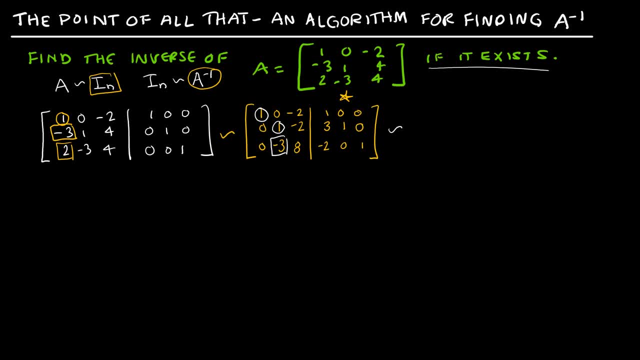 next move is to turn that negative 3 into a 0.. So row 1 will remain the same. Whoa, be very careful with your signs. You don't want to have to keep doing this problem over and over. Row 2 will remain the same. 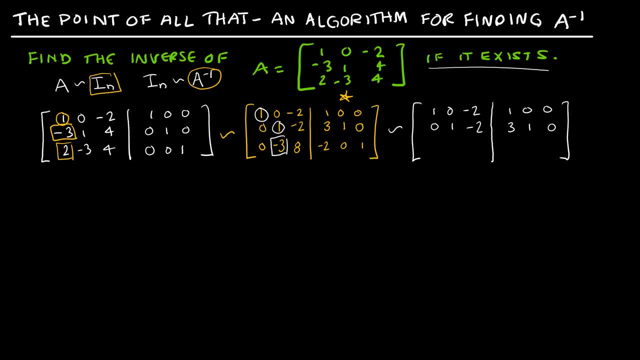 And row 3, I'm going to take row 2 times 3 and add it to row 3.. So 0, 3 times 1 is 3, plus 3 is 0.. 3 times negative 2 is negative 6, plus 8 is 2.. 3 times 3 is 9, plus negative 2 is. 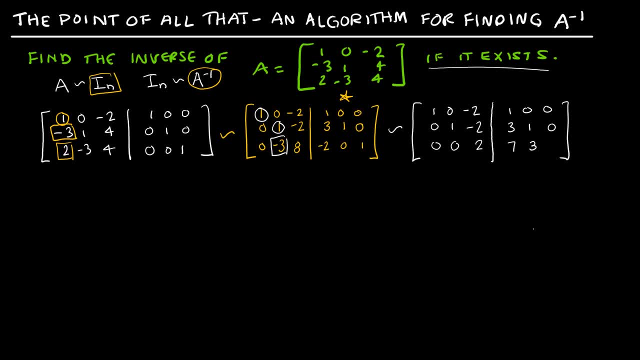 7.. 3 times 1 is 3, plus 0 is 3.. 3 times 0 is 0, plus 1 is 1.. Sorry if my mental math is annoying to you. I have to say it out loud or I will mess up. 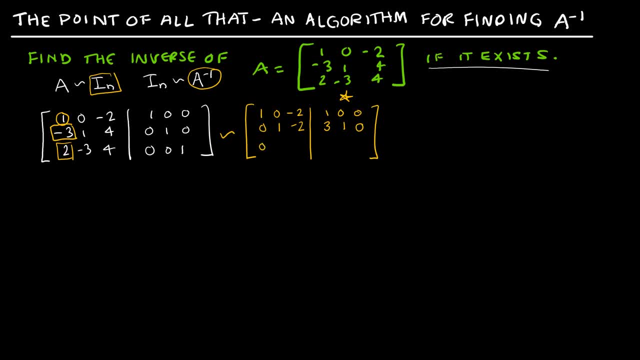 So negative: 2 plus 2 is 0.. Negative 2 times 0 is 0,, plus negative: 3.. Positive: 4 plus 4 is 8.. Negative: 2 plus 0 is negative 2. 0 plus 0 is 0, and 0 plus 1 is 1.. 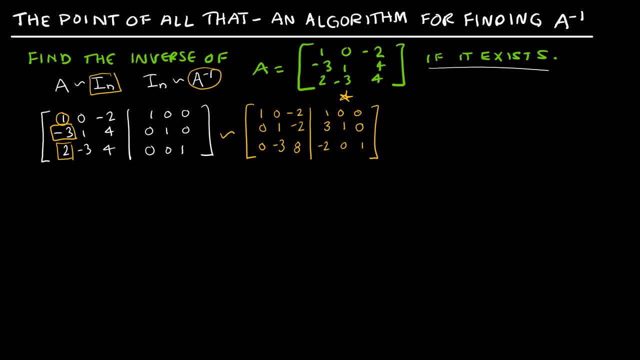 So far, so good. I have a pivot right here and I've got a pivot right here, So obviously my next move is to turn that negative 3 into a 0.. So row 1 will remain the same. Whoa, be very careful with your signs. 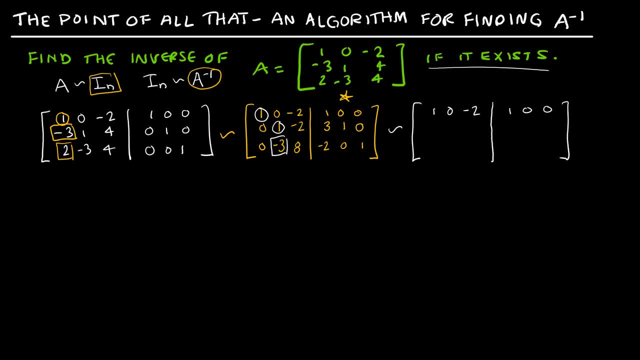 You don't want to have to keep doing this problem over and over. Row 2 will remain the same And row 3, I'm going to take row 2 times 3 and add it to row 3.. So 0, 3 times 1 is 3, plus 3 is 0.. 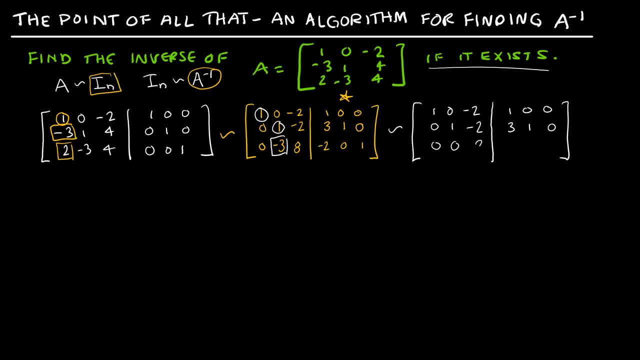 3 times negative. 2 is negative. 6, plus 8 is 2.. 3 times 3 is 9,. plus negative 2 is 7.. 3 times 1 is 3, plus 0 is 3.. 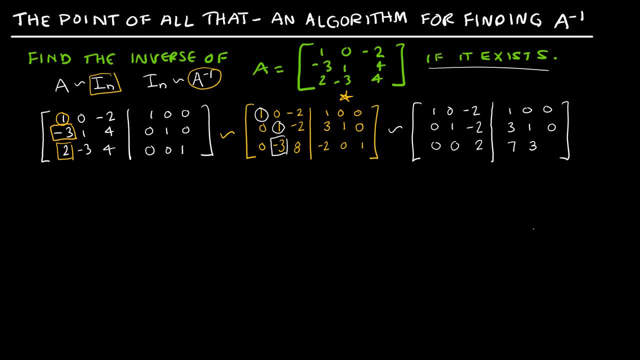 3 times 0 is 0, plus 1 is 1.. Sorry if my mental math is annoying to you. I have to say it. I'm going to say it out loud or I will mess up. Next thing. I've got one where I want it. 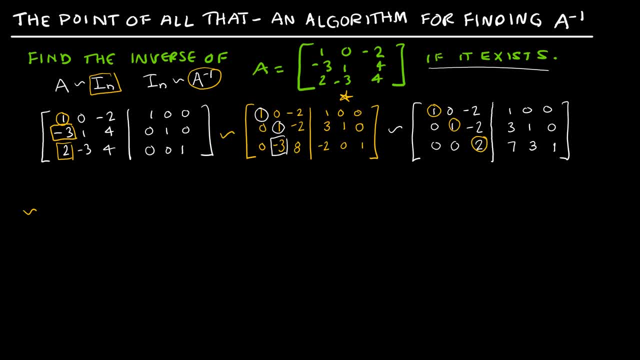 I've got one where I want it. This guy is a pivot as well. Obviously, I need to take half of everything- Sorry, half of everything- in row 3.. So row 1 remains the same. Row 2 remains the same. 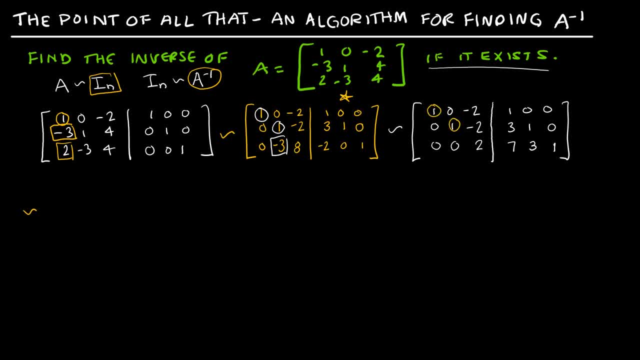 Next thing: I've got 1 where I want it. I've got 1 where I want it. This guy is a pivot as well. Obviously, I need to take half of everything in row 3.. So row 1 remains the same. 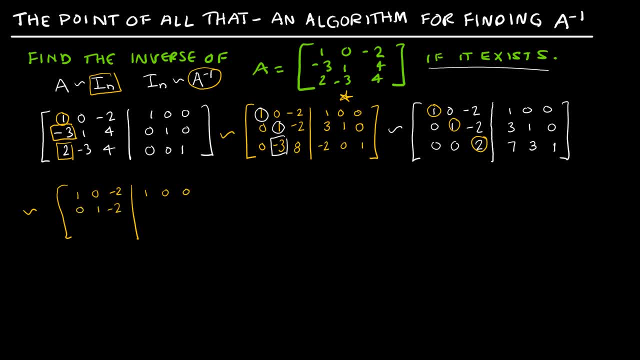 Row 2 remains the same Row 3, we go halfsies: 0, 0, 1, 7, halves 3 halves 1 half. So I've got a pivot, I've got a pivot. I've got a pivot I need for my values here and here. 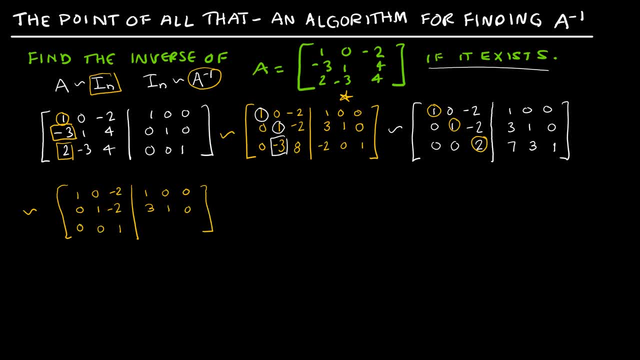 Row 3, we go halfsies: 0, 0, 1.. 7 halves, 3 halves, 1 half. So I've got a pivot, I've got a pivot, I've got a pivot. I need for my values here and here to become 0s. 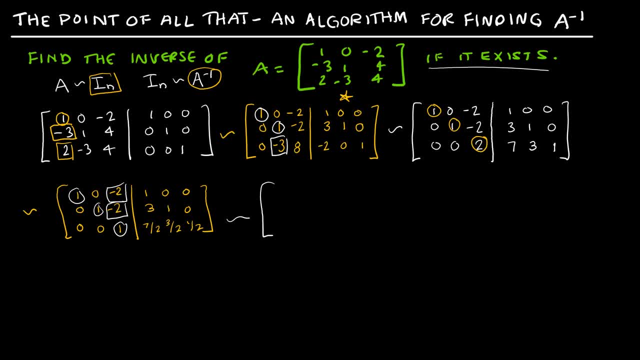 So that is my next thing. So I'm going to take 2 times row 3 and add it to row 1.. So 2 times 0 plus 1 is 1.. 2 times 0 plus 0 is 0.. 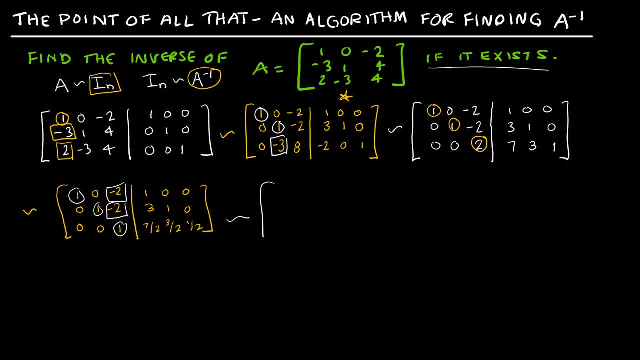 to become zeros. So that is my thing. So I'm going to take 2 times row 3 and add it to row 1.. So 2 times 0 plus 1 is 1,. 2 times 0 plus 0 is 0,. 2 times 1 plus negative 2 is 0.. That's what I. 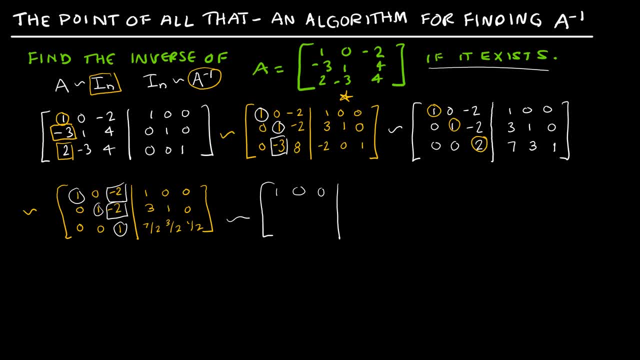 wanted Continue. 7 halves times 2 is 7 plus 1 is 8.. 3 halves times 2 is 3 plus 0 is 3, and 1 half times 2 is 1 plus 0 is 1.. I'm going to do the same to row 2.. 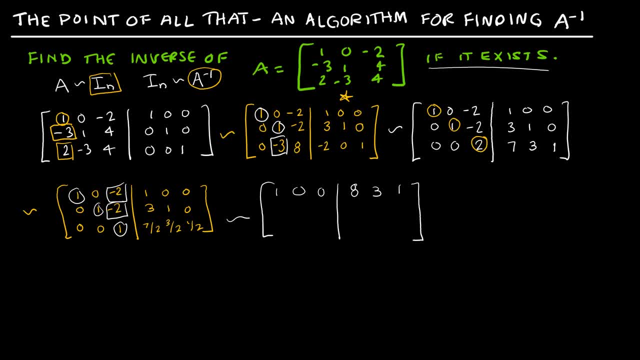 So 2 times row 3 plus row 2.. 0 plus 0 is 0,, 0 plus 1 is 1,, 2 plus negative 2 is 0.. 7 plus 3 is 10,. 3 plus 1 is 4, and 1 plus 0 is 1.. 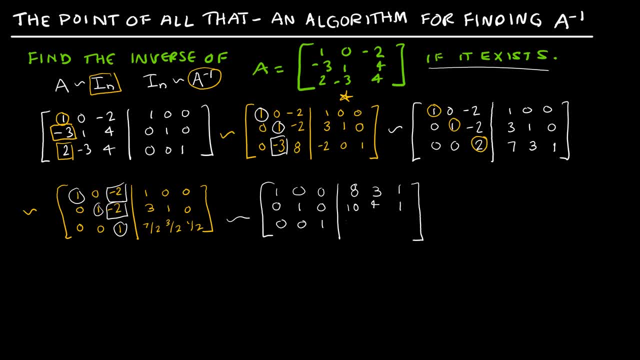 This one is already where I want it. So, unless I made a glaring mistake, this is now the identity and this is now a inverse. So let's go back up here where we talked about it before. A became the identity, The inverse became: I'm sorry. 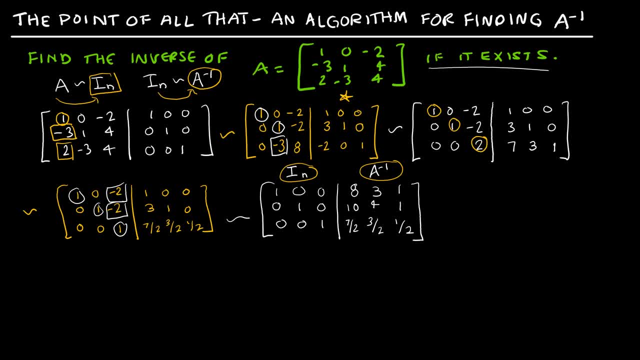 the identity became a inverse. So now the question is: did I do it right? Is that in fact the inverse? How do I know? Well, obviously I could use some technology to check it or to actually calculate it from the beginning. but where is the fun in that? If I take A 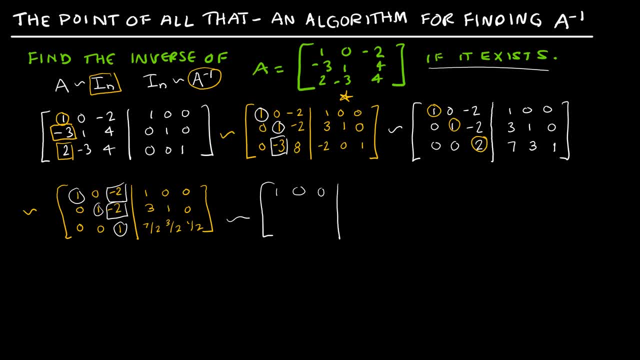 2 times 1 plus negative 2 is 0.. That's what I wanted. Continue. 7 halves times 2 is 7 plus 1 is 8.. 3 halves times 2 is 3 plus 0 is 3.. 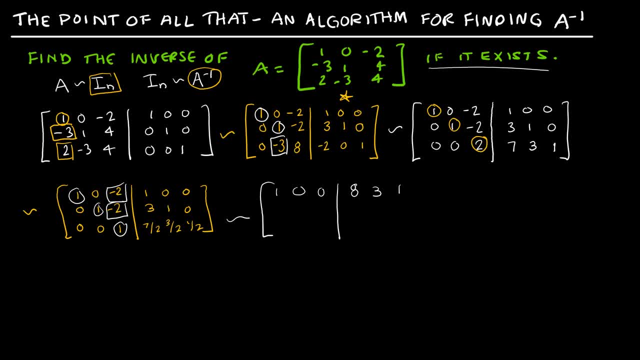 And 1 half times 2 is 1 plus 0 is 1.. I'm going to do the same to row 2.. So 2 times row 3 plus row 2.. 0 plus 0.. 0 is 0.. 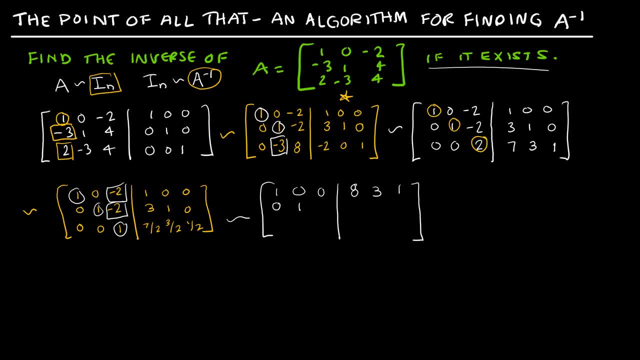 0 plus 1 is 1.. 2 plus negative 2 is 0.. 7 plus 3 is 10.. 3 plus 1 is 4.. And 1 plus 0 is 1.. This one is already where I want it. 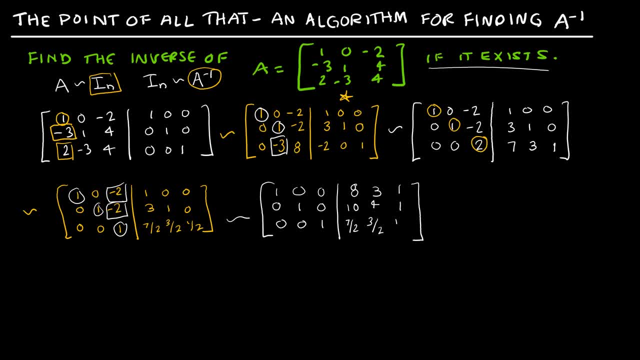 So, unless I made a glaring mistake, this is now the identity and this is now A inverse. So let's go back up here where we talked about it before. A became the identity, The inverse became- I'm sorry, the identity became A inverse. 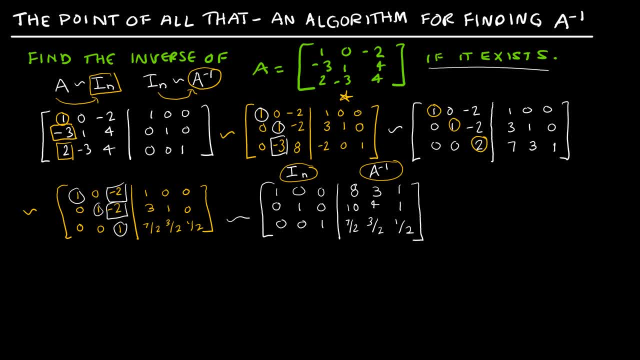 So now the question is: did I do it right? Is that in fact the inverse? How do I know? Well, obviously I could use some technology to check it or to actually calculate it from the beginning. But where is the fun in that? 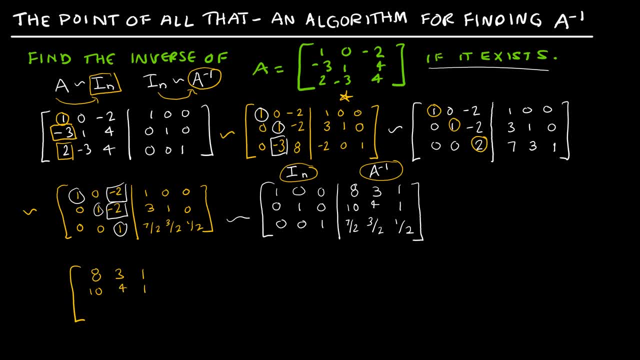 If I take A inverse times A, I should end up where? Big question: where should I end up? Of course, I should end up back at the identity. So if I did everything correctly- and I'm going to double check my signs before I multiply- 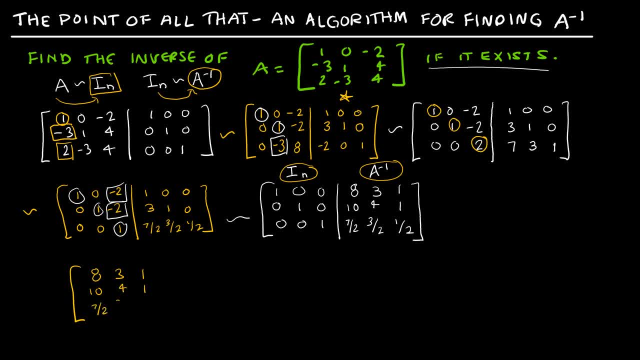 inverse times A. I should end up where. Big question: Where should I end up? Of course, I should end up back at the identity. So if I did everything correctly- and I'm going to double check my signs before I multiply- 8,, 3, 1,, 10,, 4, 1, 7 halves, 3, halves 1, half 1, 0, negative 2, yep. 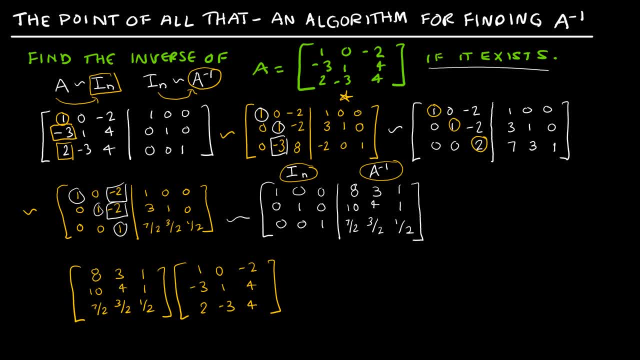 8,, 3,, 1, 10,, 4,, 1, 7 halves, 3 halves, 1 half, 1, 0, negative 2, yep, yep, yep. Okay, if I did everything right. 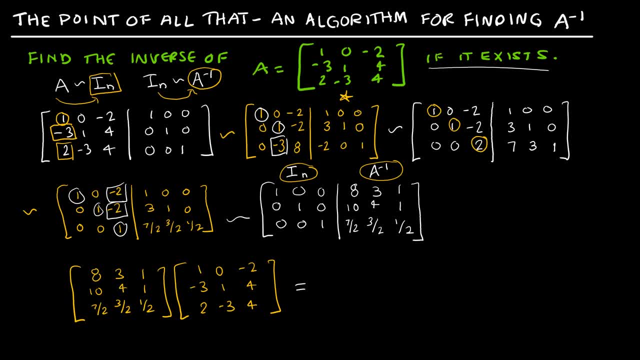 then when I multiply this, I should end up at the identity. So let's see if I know what I'm talking about. Let's take 8 plus negative 9, which is negative 1,, plus 2,, which is positive 1.. 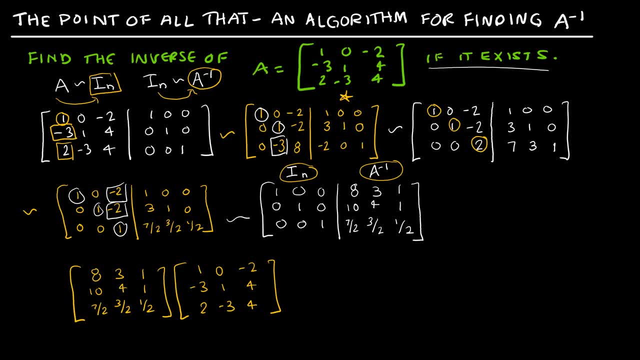 yep, yep. Okay, If I did everything right, then when I multiply this, I should end up at the identity. So let's see if I know what I'm talking about. Let's take 8 plus negative 9, which is negative 1, plus 2,, which is positive, 1.. Whew, good thing. so 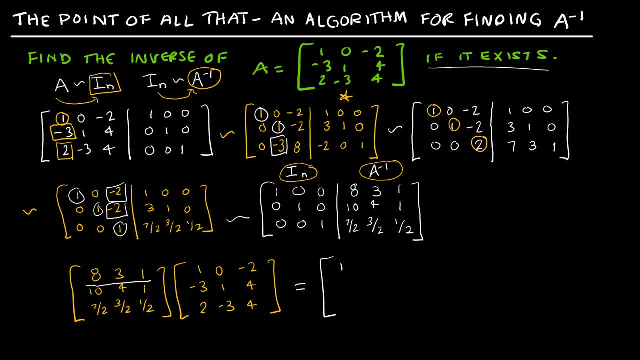 far, And then 0 plus 3 plus negative 3 is 0. And then negative 16 plus 12 plus 4 is 0.. So far I'm pretty excited: 10, 4,, 1.. So I get 10 plus negative 12,, which is: 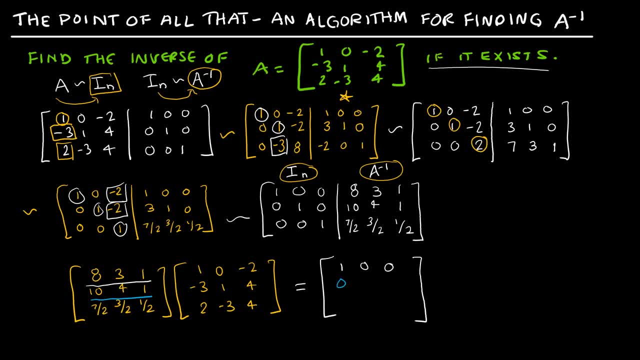 negative 2, plus 2,, which is 0. And I get 0 plus 4 plus negative 3,, which is 1.. And I get negative 20 plus 16,, which is negative 4, plus 4, which is 0.. Whew, I'm pretty stoked guys. Last one, Lots of. 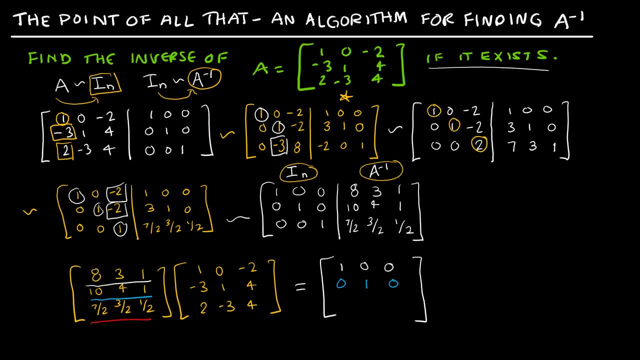 fractions. Let's see how my mental math holds up: 7 halves plus negative 9 halves is negative 2 halves. or negative 1, plus positive 1, which is 0.. 0 plus negative 9 is 3 halves. plus negative 3 halves is 0.. And negative 7 plus 6 is negative 1, plus. 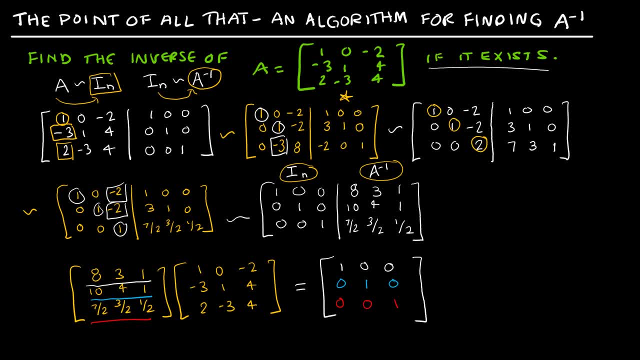 2 is positive. 1. I'm the smartest person alive. It's okay to give yourself a pat on the back. So what do I have here? I have the identity matrix, because I took A inverse times A. I did it. 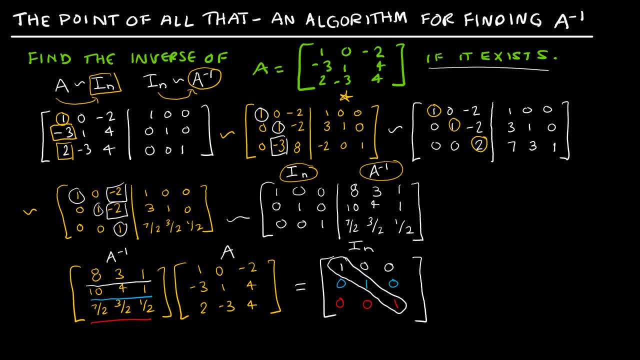 Which means my solution for all of that A inverse is this side of the matrix, which is, of course, 8, oops, let's make that a better 8.. 8, 3, 1, 10, 4, 1, 7 halves, 3 halves. 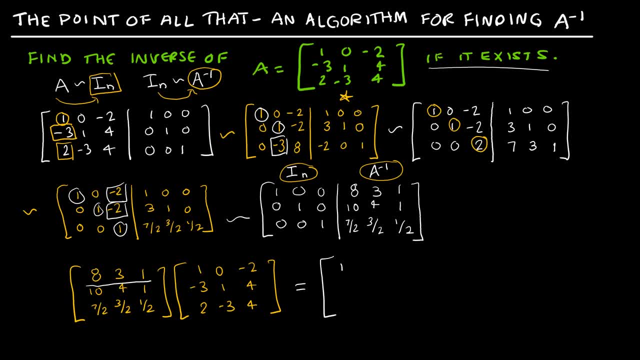 Whew, good thing so far. And then 0 plus 3 plus negative 3 is 0. And then negative 16 plus 12 plus 4 is 0.. So far I'm pretty excited: 10,, 4,, 1, so I get 10 plus negative 12,. 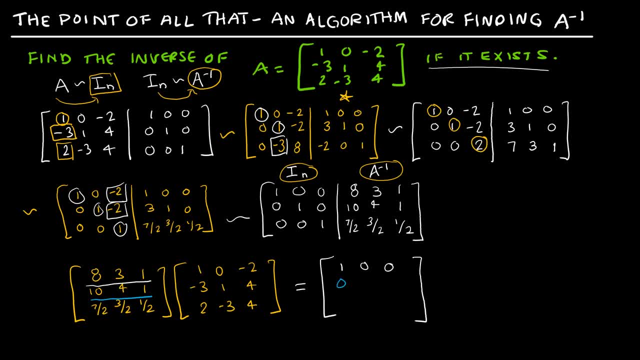 which is negative 2, plus 2,, which is 0.. Then I get 0 plus 4, plus negative 3,, which is 1.. And I get negative 20 plus 16,, which is negative 4, plus 4, which is 0.. 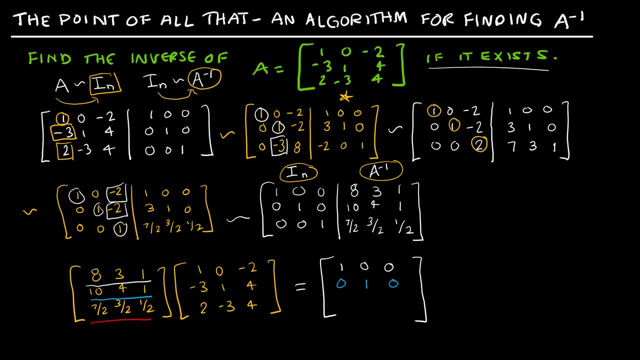 Whew, I'm pretty stoked, guys. Last one: Lots of fractions. Let's see how my mental math holds up: 7 halves plus negative 9 halves is negative 2 halves, or negative 1, plus positive 1,, which is 0.. 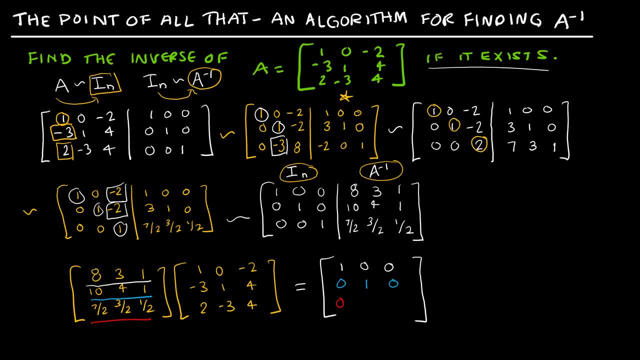 0 plus 3 halves plus negative 3 halves is 0. And negative 7 plus 6 is negative 1, plus 2. So that is positive 1.. I am the smartest person alive. It's okay to give yourself a pat on the back. 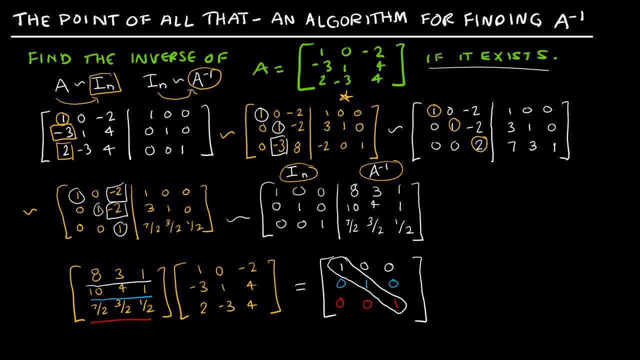 So what do I have here? I have the identity matrix, Because I took A inverse times A. I did it, which means my solution for all of that A inverse is this side of the matrix, which is, of course, 8.. 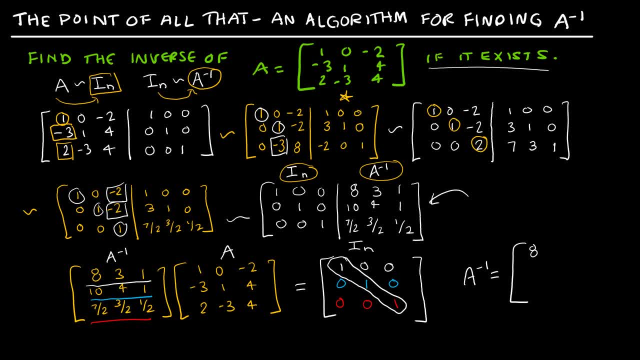 Oops, Let's make that a better: 8. 8, 3, 1, 10, 4, 1,. 7 halves, 3 halves, 1 half. I do want to point one more thing out. 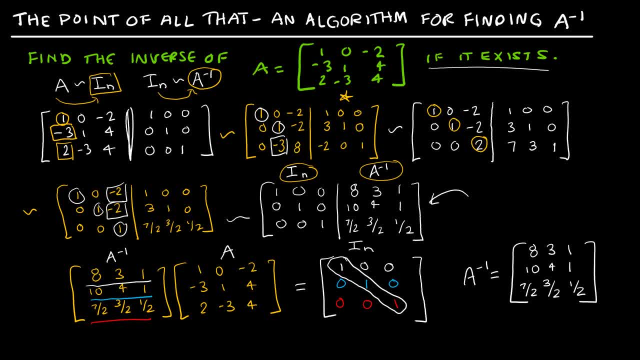 and that is in your textbook. it doesn't show this line, as it never does in our textbook, which I hate, But please do show that line. I do want to see which side is which, And I just think it makes a heck of a lot more sense. 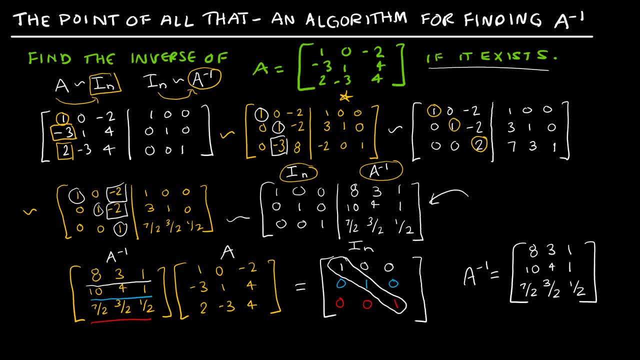 1 half. I do want to point one more thing out, and that is in your textbook. it doesn't show this line, as it never does in our textbook, which I hate, but please do show that line. I do want to see which side is which, and I just think. it makes a heck of a lot more sense.